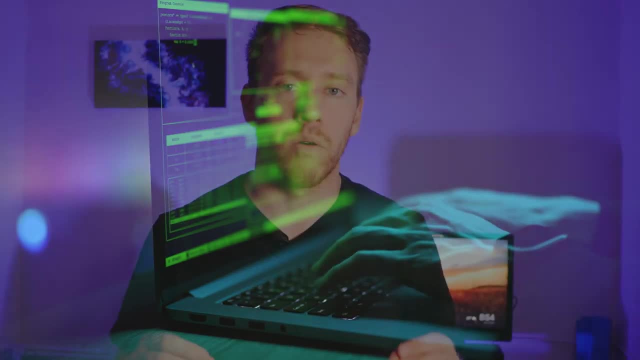 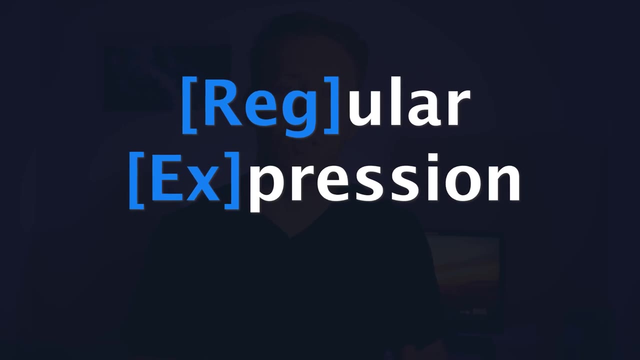 regex, and I've noticed that it is the super powerful tool in my arsenal. What is regex? Regex is a way to perform powerful pattern matching and search and replace on strings of text, and it really can be used in a wide range of different scenarios. So in this video we're not 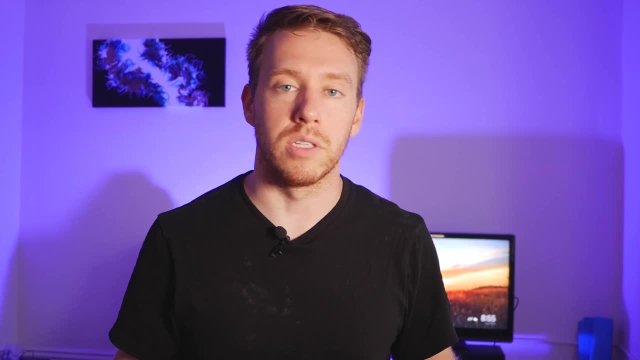 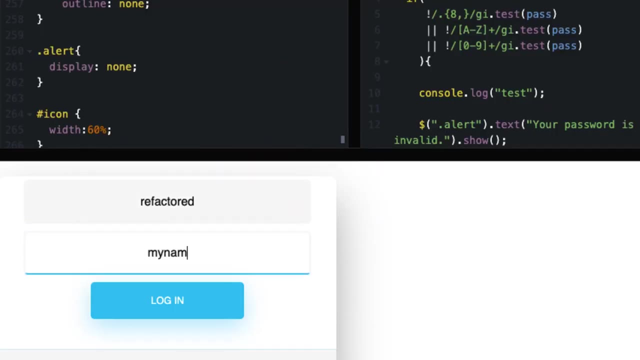 only going to lay out how regular expressions work and the definitions and how to build them, but we're going to show you tons of real life examples, like password validation or web scraping, so you're really going to understand how this works in action. This is one of those videos. 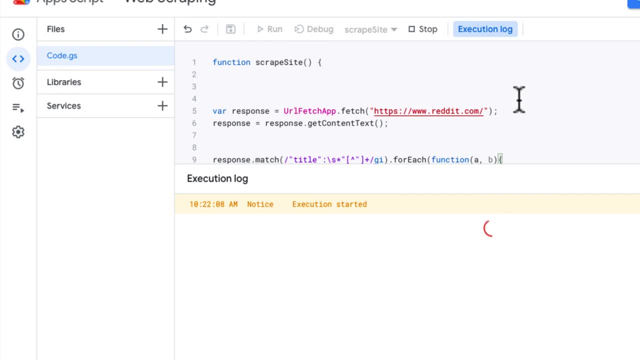 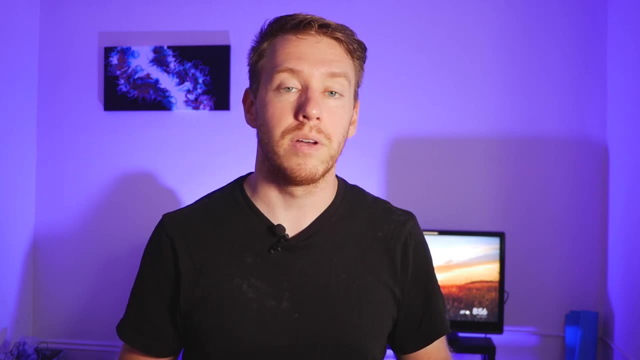 that if you put some upfront investment and watch the entire video, this is going to save you tons of time in the future, because it's going to accelerate your ability to develop at a faster pace. Anyways, let's get started. Okay, so we're going to start off using a publicly available regex. 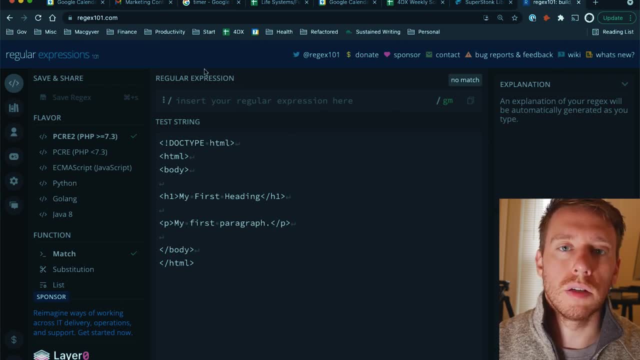 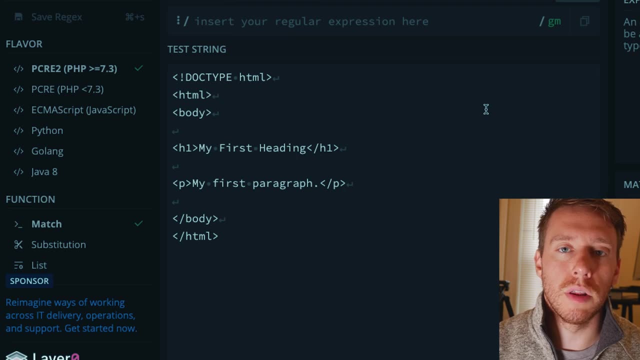 validator and towards the end of this video we're going to actually use python and javascript to show real world implementations of regex. but just to get you acquainted with the terminology and all the different syntax and patterns, we're going to use one of these validators here Now. keep in mind that every major runtime has a regex engine and they're all very similar. I would say they're subtle different flavors between them, but I would say they utilize 95% of the same exact syntax. So if you learn regex in one language, you're really learning it in all the languages. 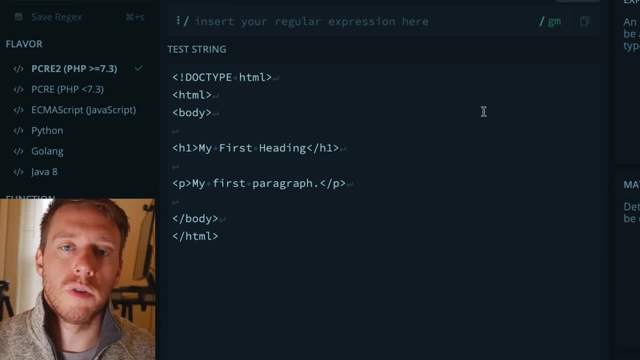 So the first thing is a regular expression is denoted by two forward slashes and you put your pattern between them. To the right of the second forward slash is the modifiers, or flags, which will introduce global rules to the entire regex. For instance, i is a flag that says: 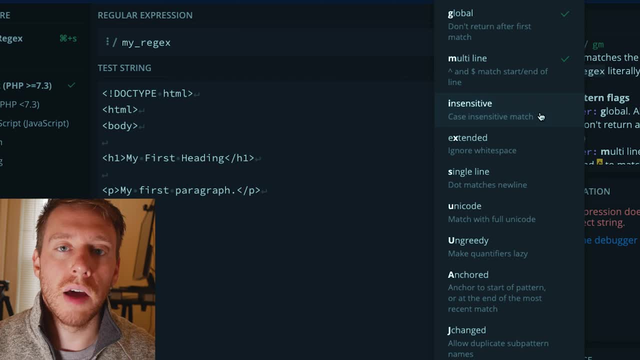 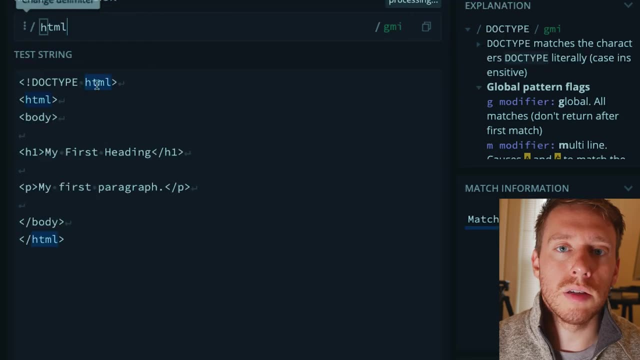 make the entire regex case insensitive, And we'll go over the remaining flags later in the video. So one thing I want you to keep in mind is that a string is also a regex. It's just an exact search regex. So if I type HTML into the regular expression, it will match on all instances. 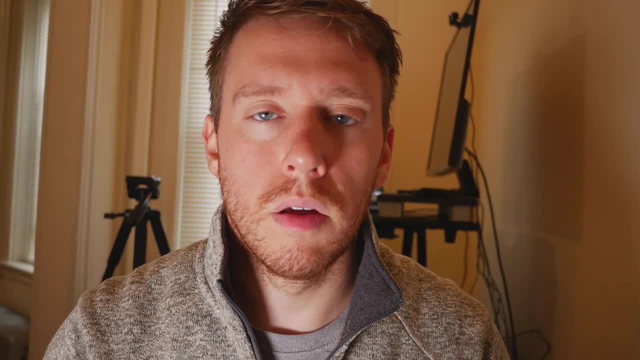 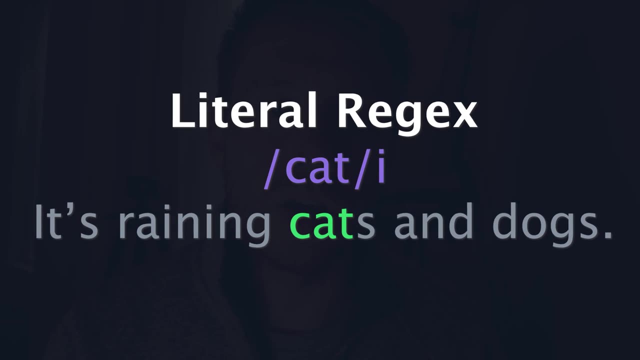 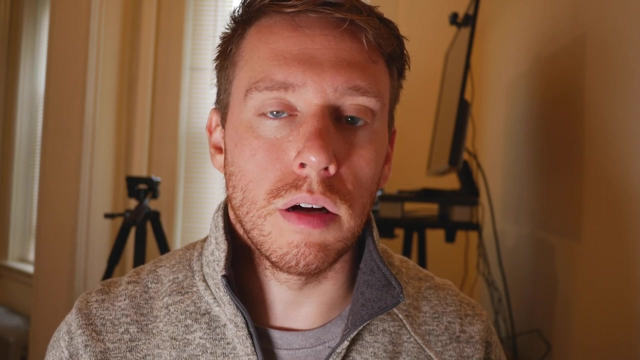 of HTML and it will be case sensitive. So when we do this, we're using literal characters. When I type in H, I'm literally looking for another H. These are called object literals. In addition to the literal characters, there's a special set of meta characters called special characters. 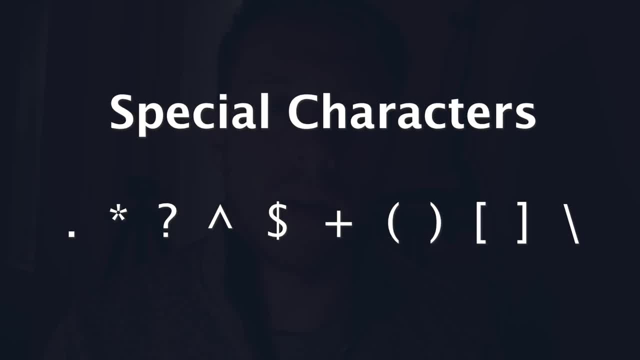 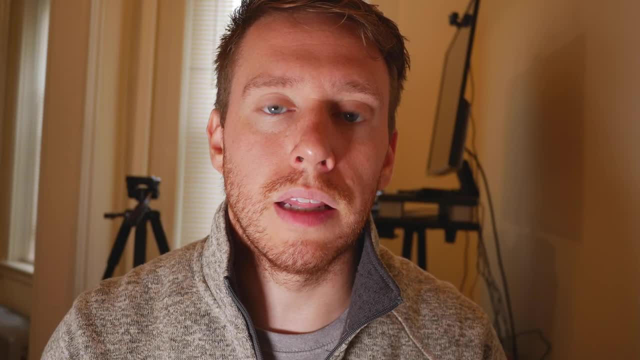 which have a specific meaning, And when you type them into a regular expression, you don't actually look for those characters. You're looking for something more generic. So we're going to start by looking at the various meta characters. So the first and most powerful meta character is the dot. 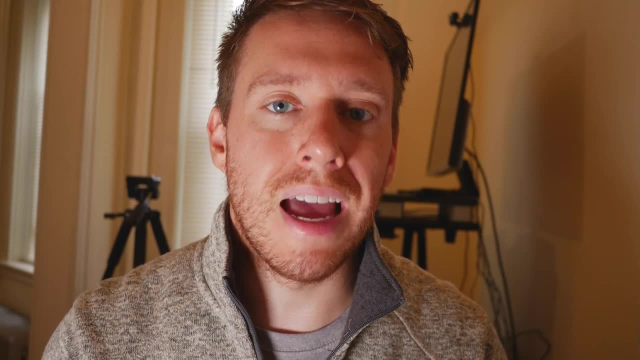 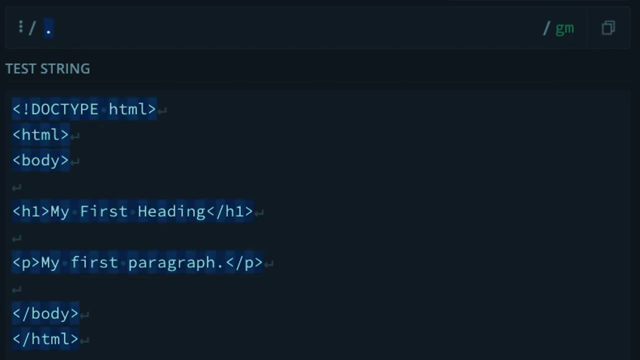 The dot will match on a single instance of any character. So it is the most broad generic regular expression that you're going to have at your disposal. So if I go ahead and type in a dot here, you will see it matching on every character. So the next meta character is the question mark. 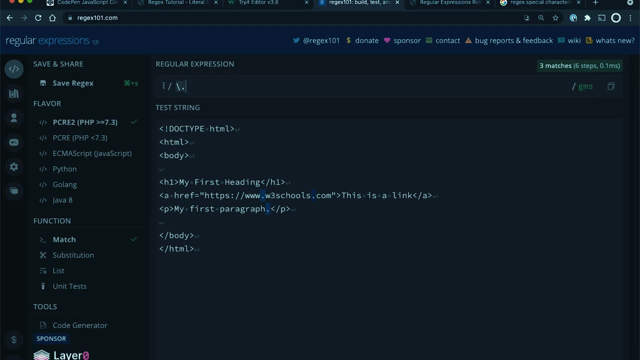 The question mark says: for any pattern that is followed by a question mark, make the pattern optional. And this is useful if we want to match on a pattern that that might contain a character or a substring and we're not sure. So, for instance, in this example, 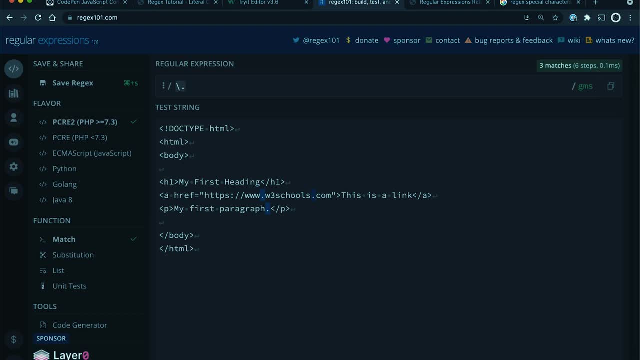 we're going to match on a character, but we're not sure, So we're going to match on a sub string. For example, say, we want to match on both open and closing HTML tags. Well, closing HTML tags have a forward slash in them and the open do not. 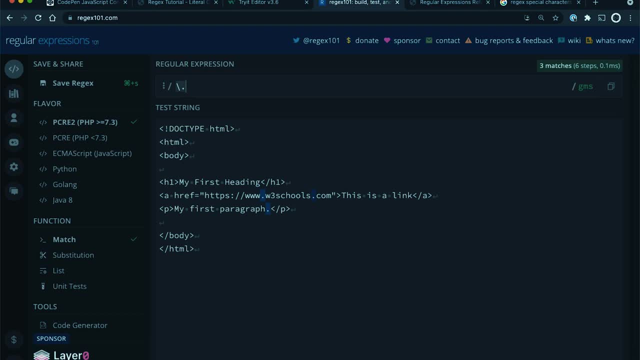 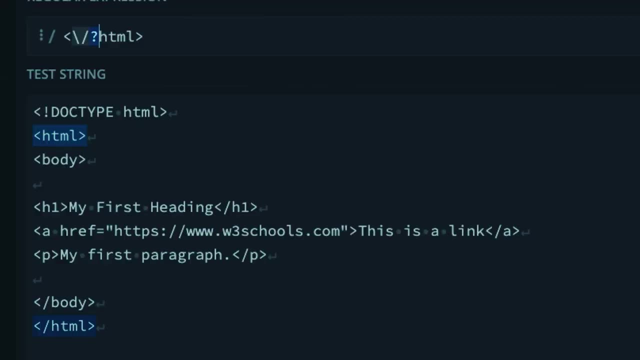 So we can utilize the optional character in order to match on both, And so this would look like the following: And now we have a regex that is generic enough to match on both open and closing HTML tags. Next we have the pipe, and the pipe just says or: 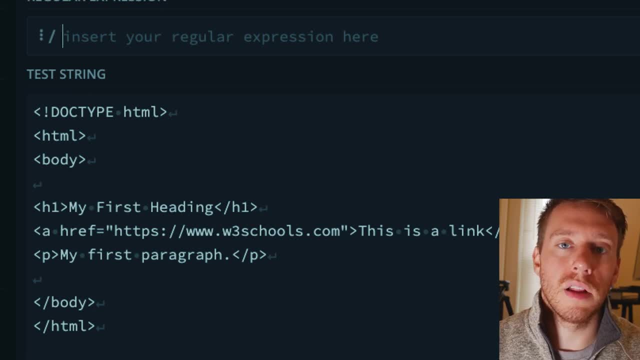 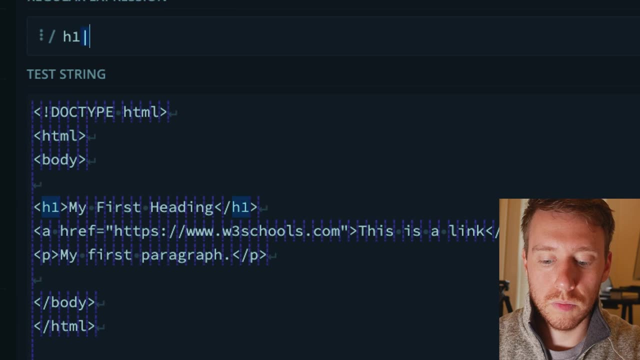 So say, we wanted to match on two terms. we could just put the first term to the left of the pipe and the second term to the right of the pipe, And now we'd match on both instances of the string. Now you can see that we're matching on instances of H1 and instances of HTML as well. 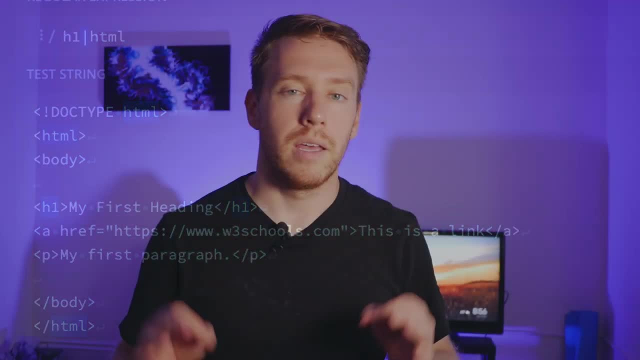 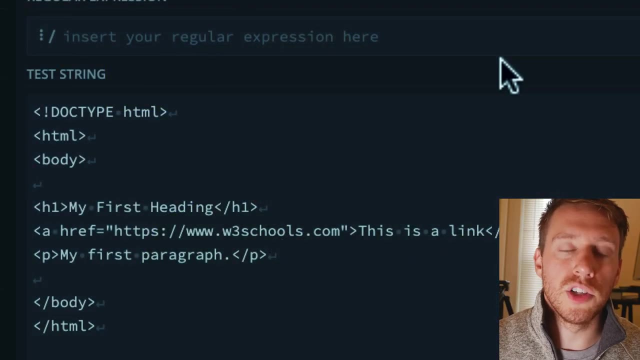 And we can continue to expand that sequence as long as we'd like. If you're liking this video, go ahead and turn that like button blue so we can get out to a wider audience, Thank you. So now I want to talk about regex shorthands. 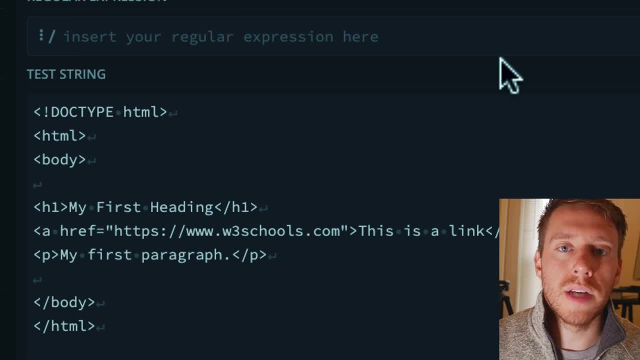 Shorthands are little sequence, regular expressions that tackle common use cases, for instance matching on a word or a digit or a space. So let me go ahead and show you those. So the first one is: to match on a letter is backslash W. 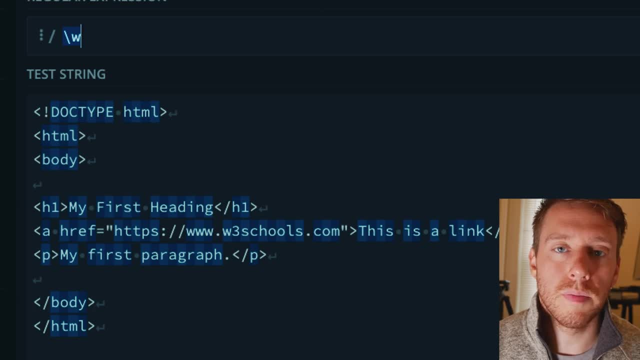 So now you can see we're matching on all the letters in the test string. To match on a digit is backslash D. So now we've found all the digits in the string And then to match on a space we use backslash S. 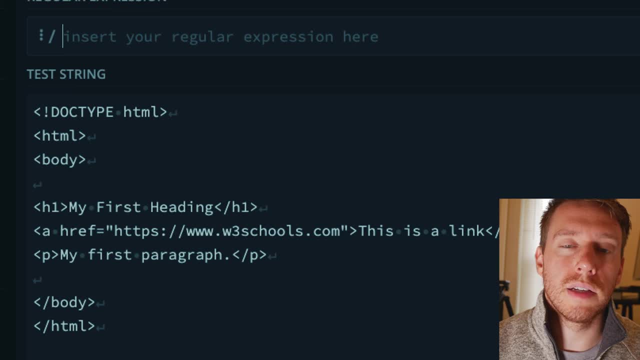 So let's talk about anchors for a second, because I find that these are pretty much necessary for writing comprehensive regular expressions. So an anchor is for any given test string. you have lines, usually, so new lines, but you also have a start of the whole blob of text, right? 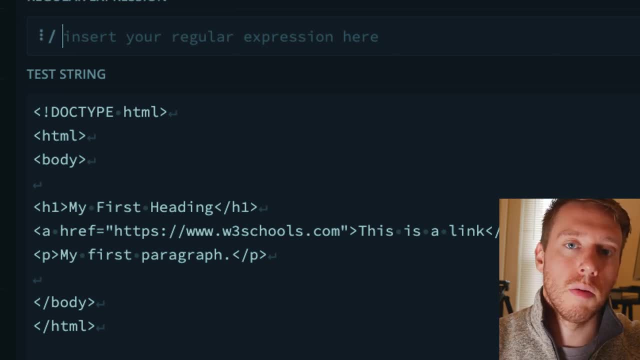 The very first character, and then you have an end of the entire blob of text. So how do we denote these different orientations within the test string? And the answer is: we use anchors. So the start of a line is going to be denoted by a caret. 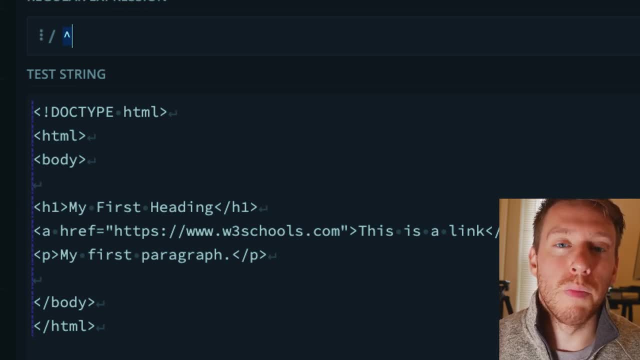 And that looks like this: The end of a line is denoted by a dollar sign, And that looks like this: The start of the entire blob of text is denoted by backslash capital, A See. that only matches once on the very start of the test string. 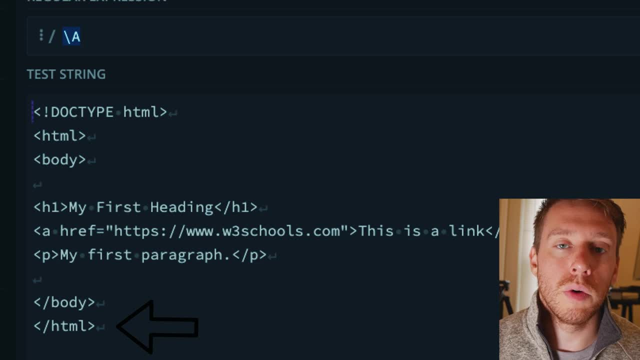 Likewise. So if we want to match on the very end of the test string, we use backslash uppercase Z. This is useful because it allows us to place the regex in a certain position, especially when the test string is very long. Take like, for example, an entire HTML document. 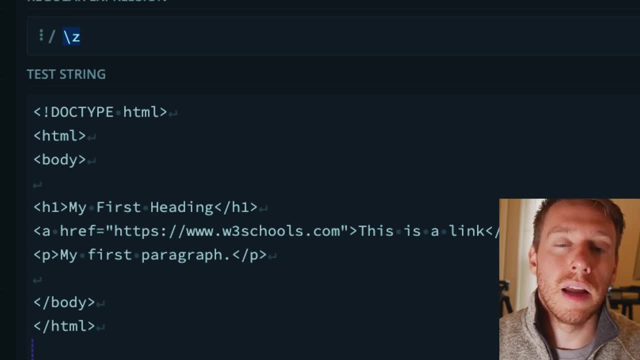 We might want to find the first or nth instance of something, And in order to do that, we need to know where we are and be anchored to the start or the end of the string. Okay, now I want to introduce a concept called repetition. 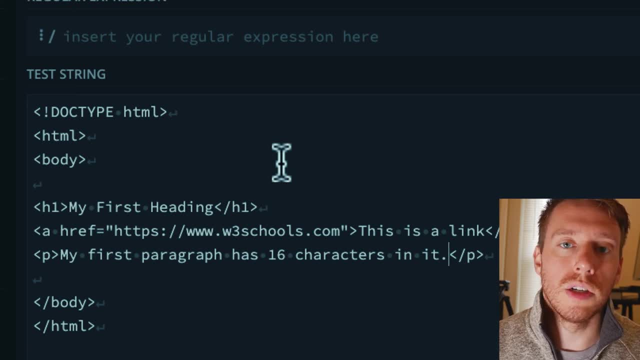 So say, for instance, I want to match on two digits. I could do that with backslash D, backslash D. but there's a more concise way to set that up. I could do one backslash D, and then I can define the number of digits that I expect. 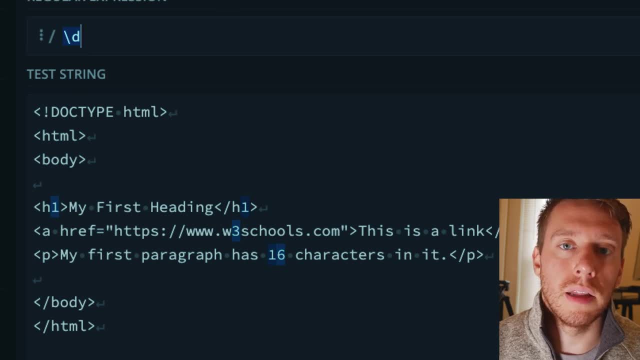 to show up, And to do this we use curly braces to indicate the number of times we want the preceding regex to appear. So I'm going to do open curly brace 2, close curly brace, And now you can see it. only matches on the 16.. 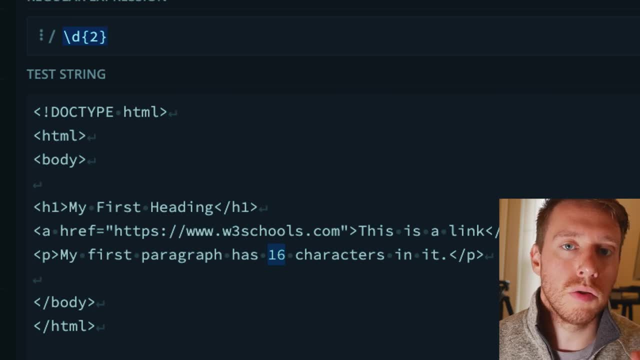 Okay, Because that's the only instance in this test string where there are two digits in sequential order. Now this repetition syntax can get even more comprehensive. We could create a range So we could say find digits that fall between a min and a max. 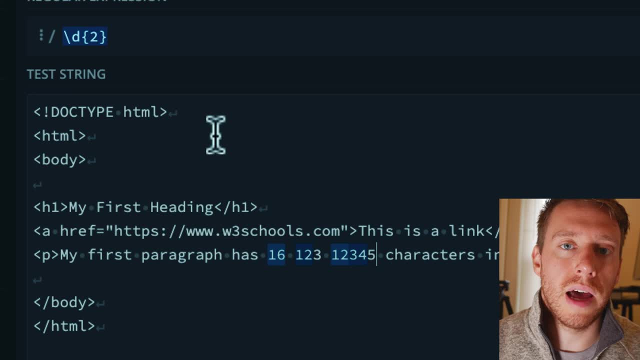 For the sake of this example. here let's find instances of digits that have at least three to five characters. So I'm going to use three for the min and five for the max. And now you can see we're matching on one, two, three. 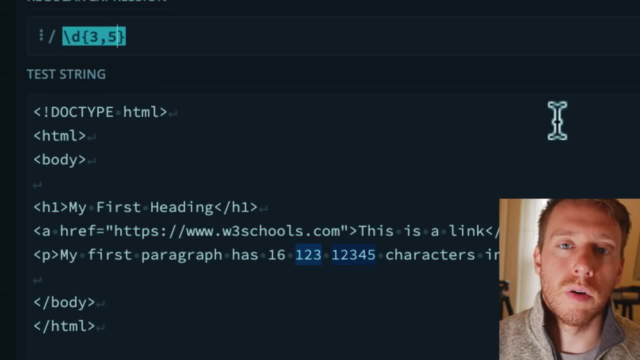 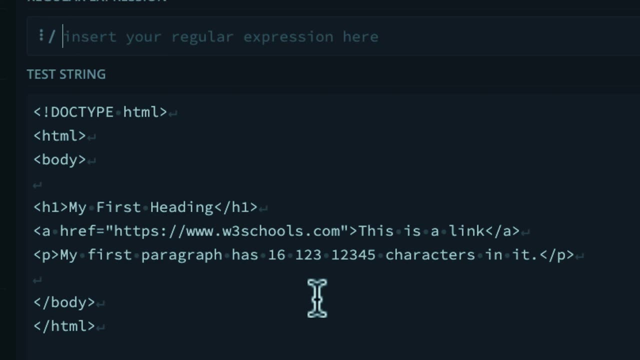 We're also matching on one, two, three, four, five. So again, these repetition functions allow us to just create more concise regular expressions. If we wanted to match on five digits, we could do the following, Or we can just do this: 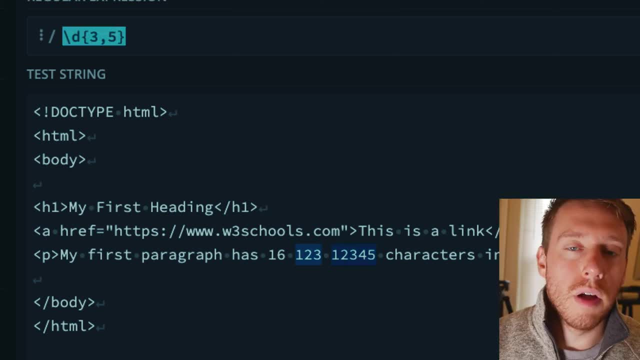 And, as you can see, this just shortens the regular expression. It's more efficient. A couple other little notes here is: if we don't want a min or we don't want a max, you can just leave it blank. Okay, If I wanted to do find digits that have three or more characters, I'll just do three comma. 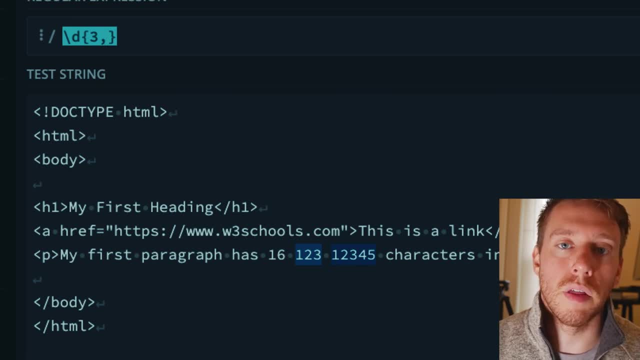 blank, And now you can see we're matching on all instances where there are three or more characters. Now, instead of using the curly braces, there are a couple shortcuts that have been made just for convenience, And the first one is the star, the asterisk. 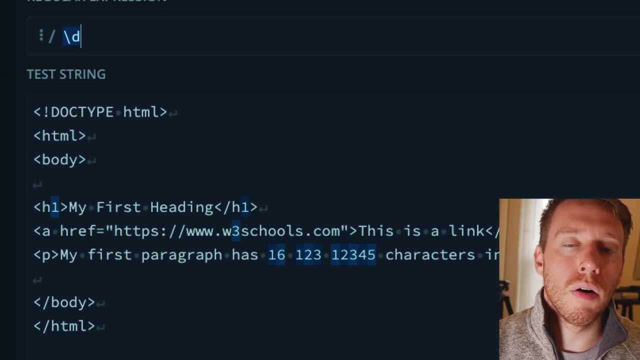 So the asterisk says that look for zero or more instances of whatever the preceding regular expression is. So if I do backslash D star, it looks for any number of digits. The next one is the plus sign. The plus sign says: look for one or more. 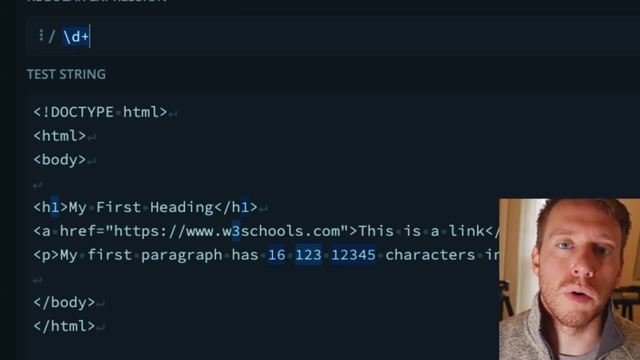 And now you can see we're matching. on all instances where there are one or more digits, The asterisk and the plus sign will usually be interchangeable, but for a small set of narrow use cases And the more generic one is the asterisk. so I'd stick to using the asterisk and you'll. 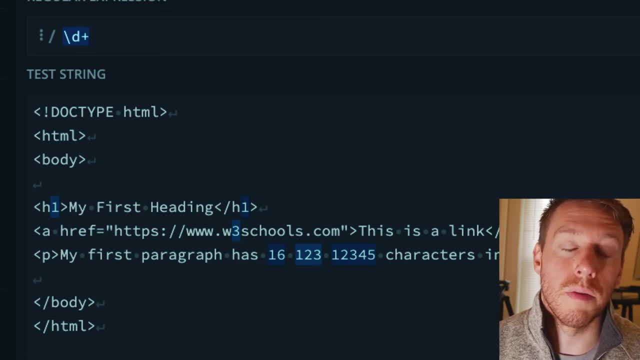 probably be good most of the time. There's just a couple scenarios where it matters if you use the asterisk or the plus sign. Okay, let's talk about capture groups. So capture groups are denoted by parentheses and they do two things. 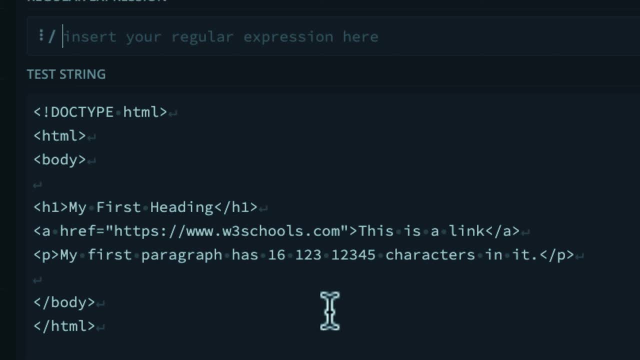 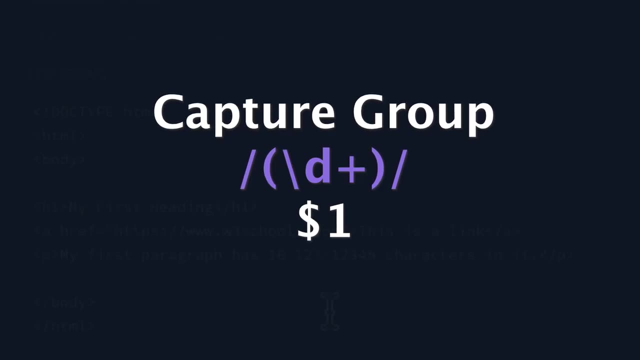 One is they allow us to create a subregex, which is very powerful. Two, they allow us to store whatever is captured in that subregex in memory so that we can reference it later, maybe for search and replace or maybe for back references. 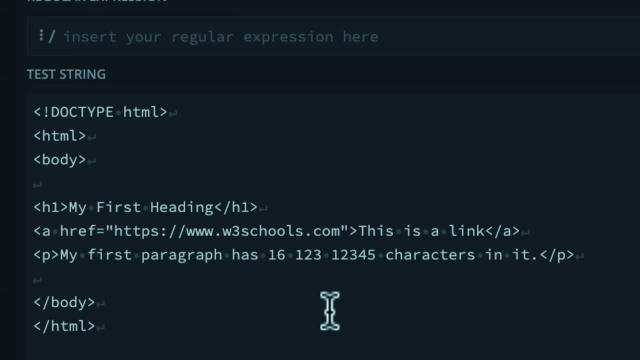 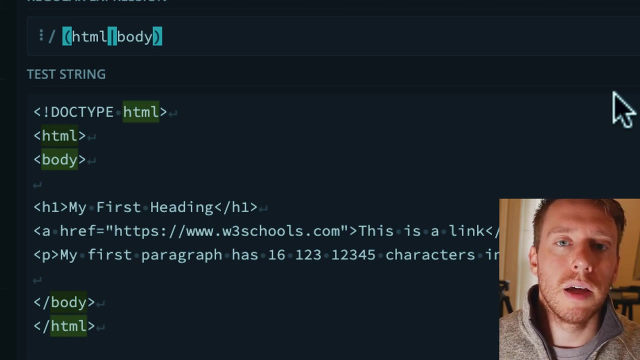 So let's create a little capture group, And you can see I use the pipe to denote those two strings. Okay, so to give you a real feel for how capture groups work, I'm going to write a regex here that matches on the h1 tag. 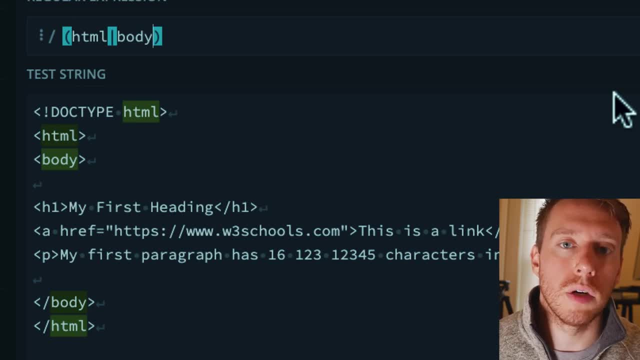 And we're going to extract the inner text of the h1 tag So you can see this regular expression is using the open h1 tag and the closed h1 tag to kind of anchor the dot star question mark which will eat up everything between those. 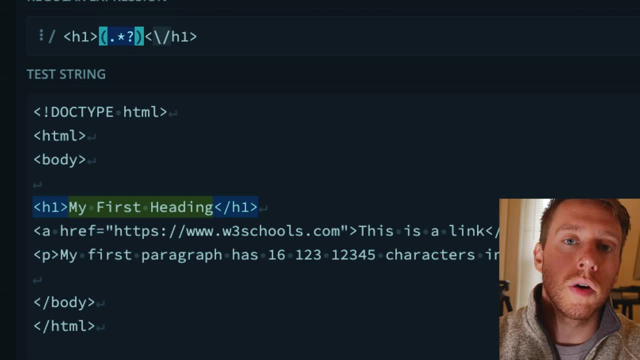 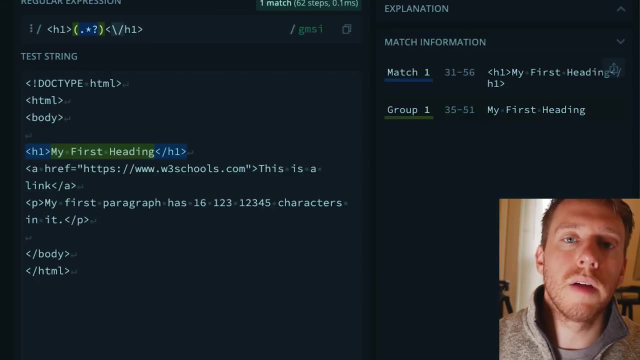 two anchors And then we use a capture group because we want to store that text in memory so that we can reference it as a capture group. So I'll show you how to do that. So if I pull out the match information here, you can see the first part. 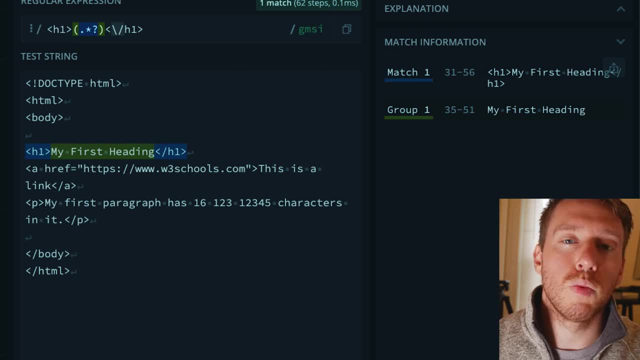 The first part is the match, which is the entire regex, But the second part is what the capture group referenced And in code, if we wanted to reference this capture group, we would do so by using dollar sign index, And in this case it's the only capture group, so it'd be dollar sign one. 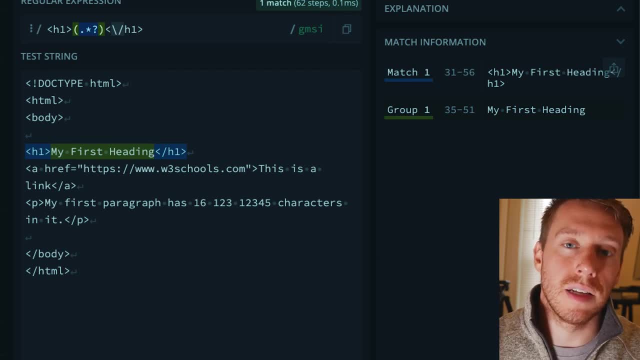 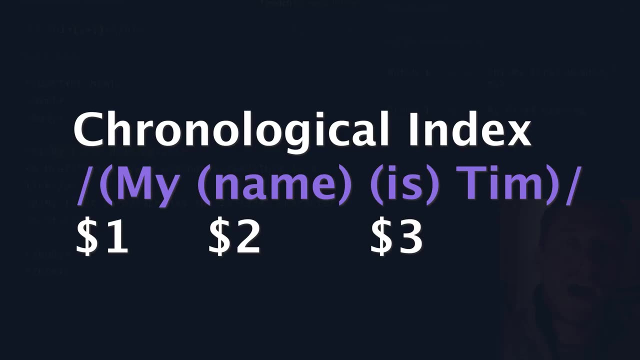 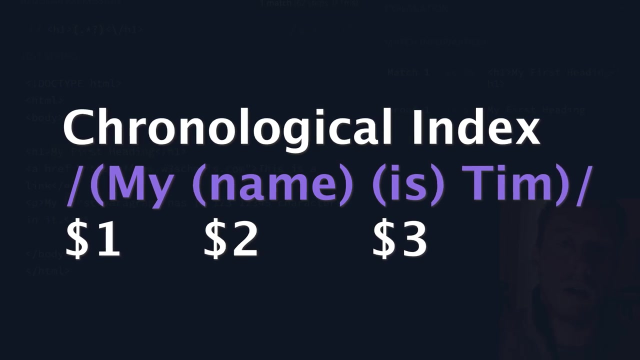 But as you build more capture groups- and you might have nested capture groups- you need to know that they are referenced based on their sequence within the regular expression and specifically the sequence of the open h1 tag, And in this case, the first part is the open parenthesis, because it's going to get very 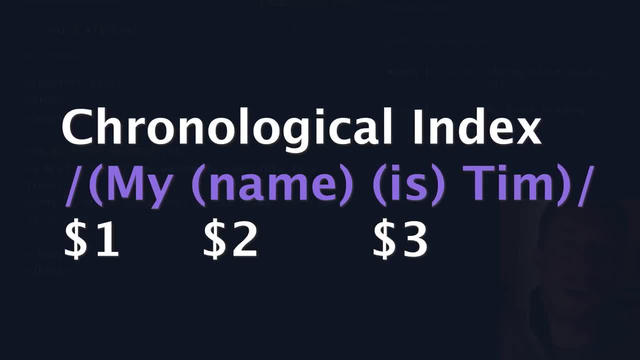 complicated, as you have nested regular expressions, But all you need to keep track of is the open parenthesis, And that will give you the index of the capture group so that you can reference it later, Say, for instance, if you're doing a replace or a text extraction function. 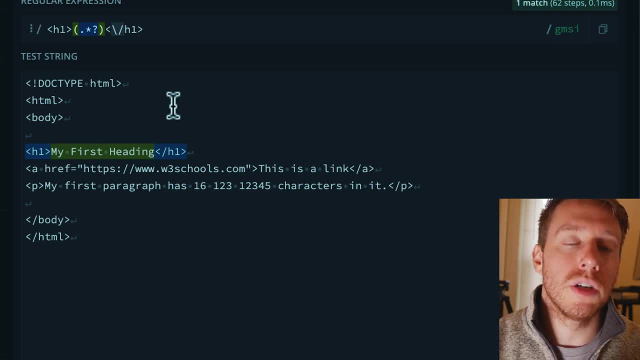 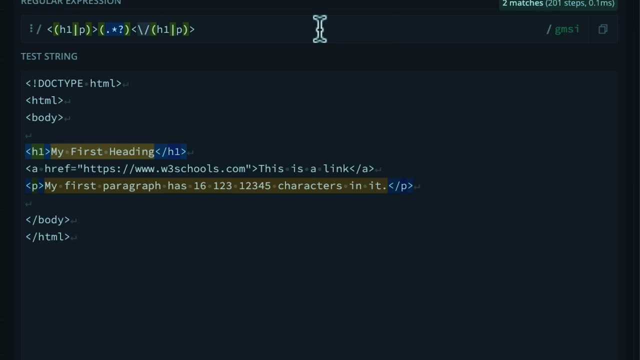 So say: I also wanted to extract the text from the paragraph tag. we can modify this regular expression to be generic enough to match on both instances. So I'm going to go ahead and do that groups and the or the pipe in order to make this regex more generic. but say, for instance: i don't 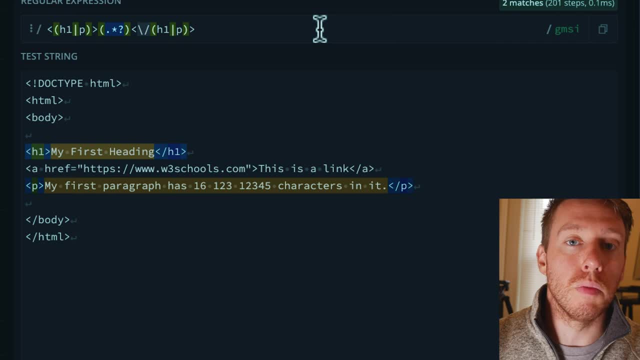 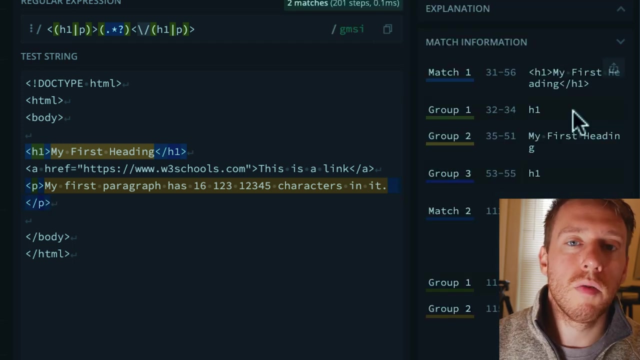 want to use the first and last capture group to store anything in memory. i just want to use them for the ability to create a sub expression. we can actually cast it to a non-capture group by using a question mark colon in the beginning of the regex. so you can see on the right all the different. 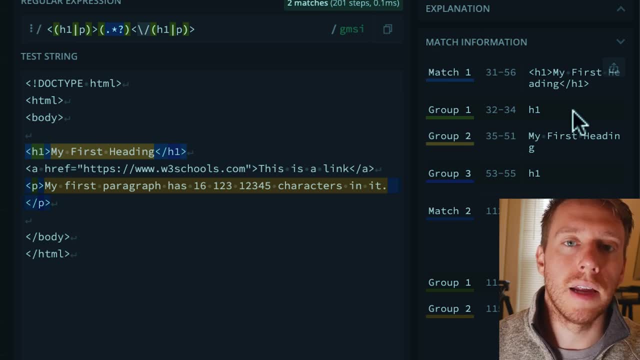 groupings that it captured. but again, we don't want to capture the tag name, we just want to capture the inner text. so we're going to use that question mark colon to convert the first and last capture group to non-capture groups. okay, and now you can see that we're only storing that. 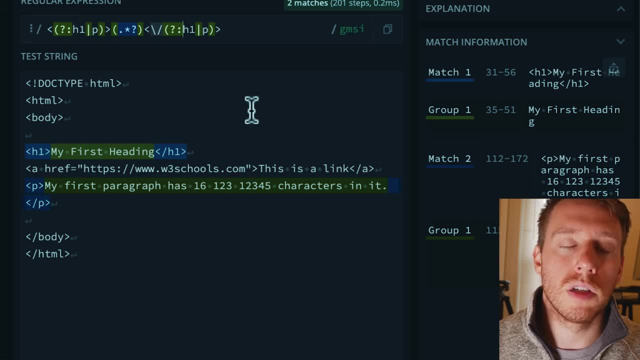 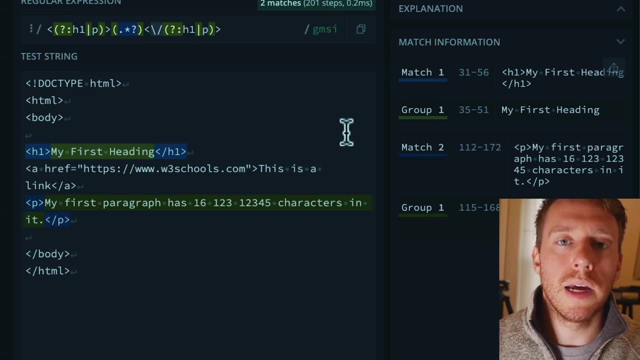 capture group that we care about in memory, and the other ones are just used for the sub-expression function. now, i don't think every regex engine supports this, but some of them do, and what you can do is, instead of using dollar sign one, you can actually name the capture group. 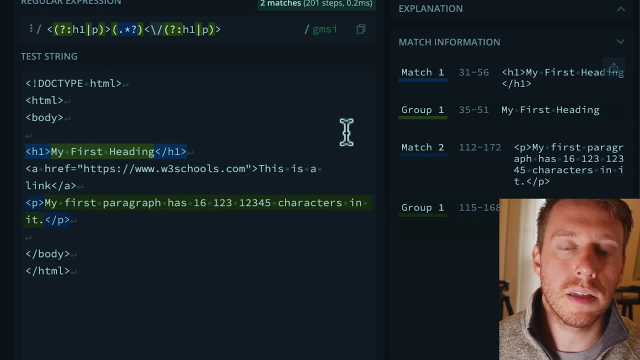 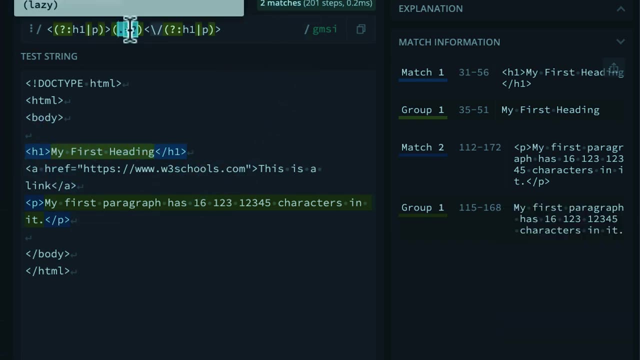 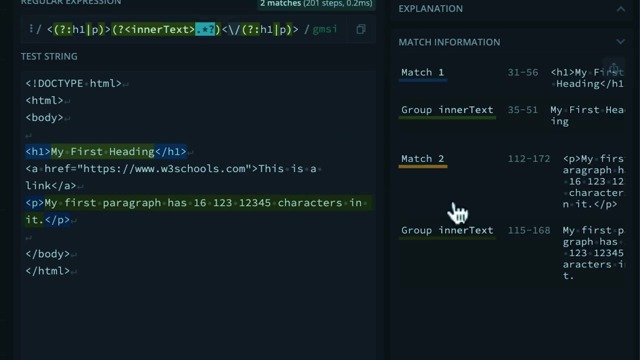 so say, for instance, we wanted to name our capture group inner text. we could just add a question mark and between two left and right arrows we can add the name, and now you can see the group is referenced by its name, not by its index. okay, now let's talk about character classes. 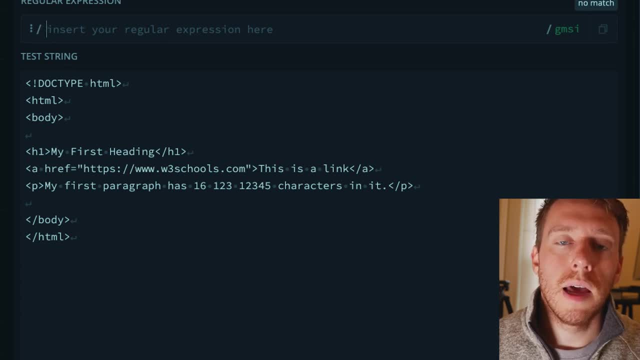 so character classes are denoted by brackets, and anything that falls within the bracket it will attempt to match on. so it's kind of a way for us to create a very generic expression. so say, for instance, i wanted to match on any letter or digit. we could do that by using the. 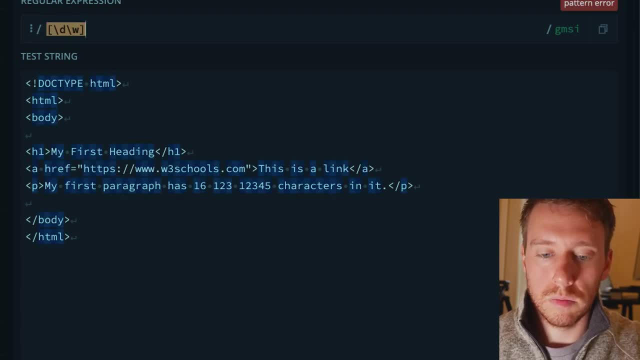 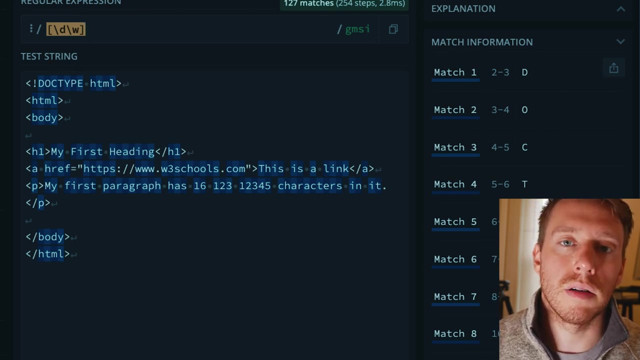 following, and again, this only matches on single instances, but say we wanted to do any number of letters or digits, we can add the repetition flag plus to say match on n number of characters or digits and then if we add the plus it will match on any number of characters or digits. 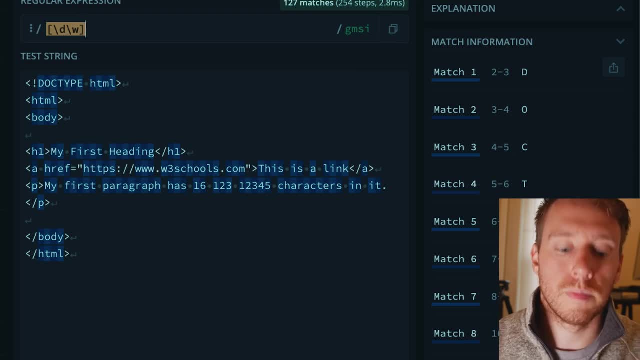 and you can see how that changes what is actually matched on now. i told you that the backslash d and the backslash w were actually shorthand, and that is true. there's actually a different way to match on digits and characters. that is sometimes useful. so if we want to match on any number of digits, you can use the range function. 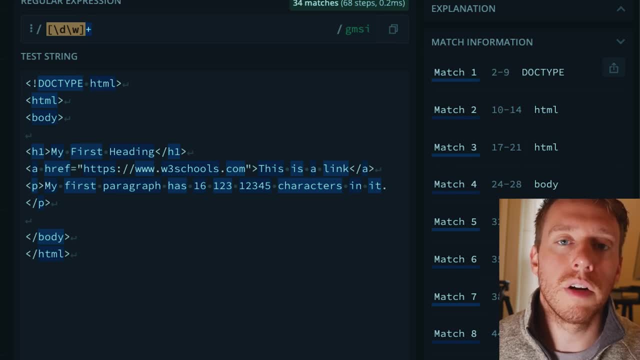 to determine which digit you want to match on. so say we want to match on zero through nine, you could do zero hyphen nine and that indicates it'll match on that entire range of digits. and intuitively, if we wanted to match on only one through five, 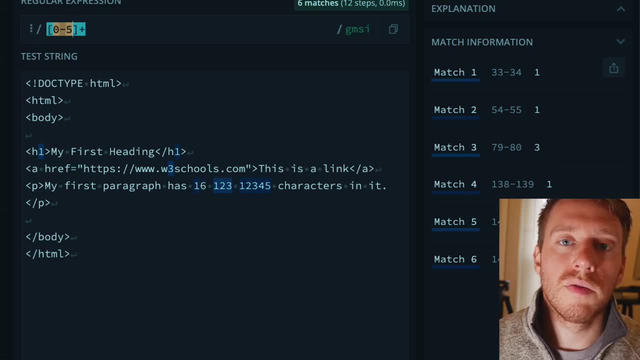 we could just create a range that indicates that, likewise for letters, you can use a range for the alphabet, so we could. if we want to match on any letter, we could just do a through z, and this will be lowercase letters if we wanted to match on uppercase as well. 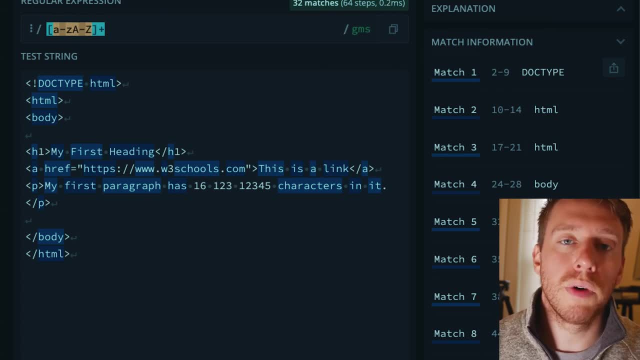 we would just do capital a through capital z. but you can also put any character in here so say: we want to match on forward slashes. we could throw those literals in here as well. we could also do spaces. we could also do something interesting which is called a negated character class. 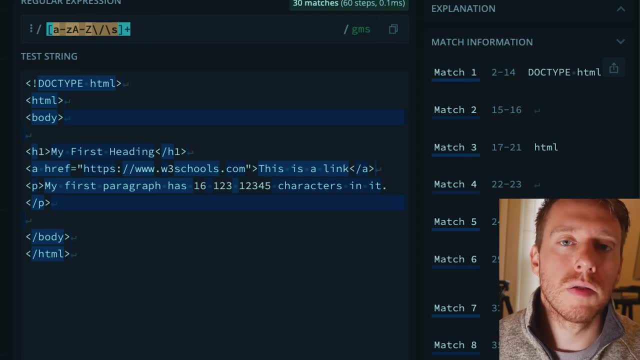 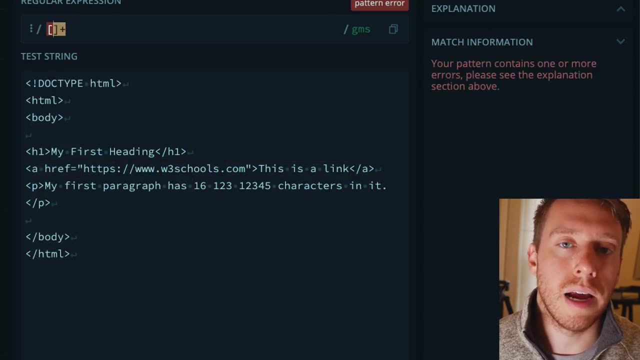 which means it will match on anything except. so say, we wanted to match on anything except a white space. so to create the negated character class, we just start with a caret, followed by the character that we're not trying to match on. so now you can see, we're matching on everything except for spaces. 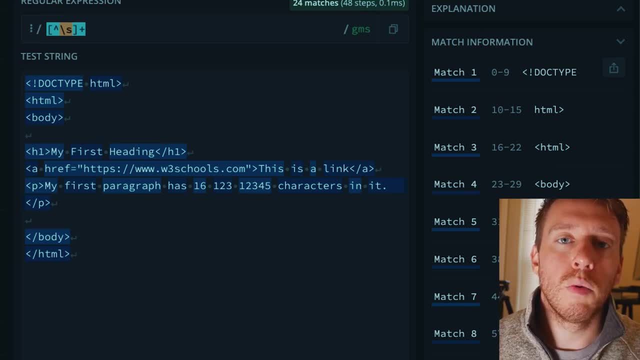 the reason negated character class are useful is because they will allow you to look for everything except the next instance of something. so in a way it functions very similar to dot star question mark. so let's actually redo the regular expression to find the inner text. but instead of using dot star question mark, let's use the negated character class. 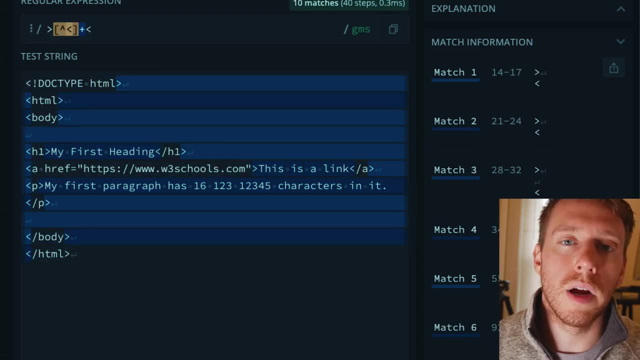 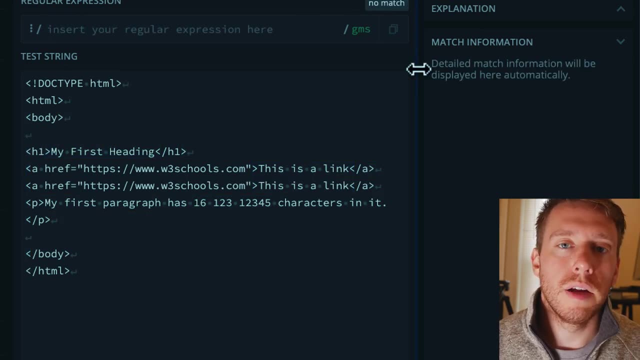 so once again, we're matching on everything between the right arrow and left arrow, but we didn't need to use the dot star in this case. so with the dot star or the dot plus, there's two concepts i want you to keep in mind. one is lazy verse, greedy, and lazy just says: find the next instance and greedy. 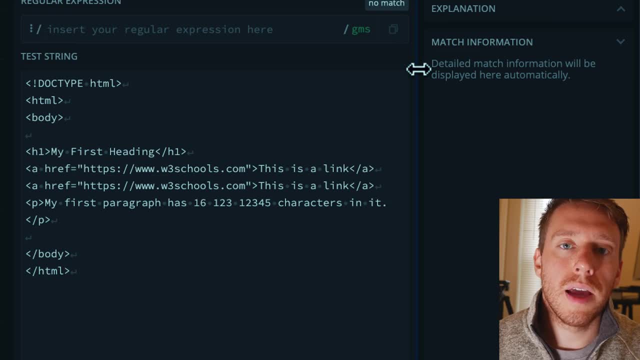 says find the last instance. so say we wanted to capture all the text leading up to the first anchor tag, we would use the lazy approach. so i'll go ahead and create that regular expression. so you can see because i use the question mark: we're capturing all the text up to the first. 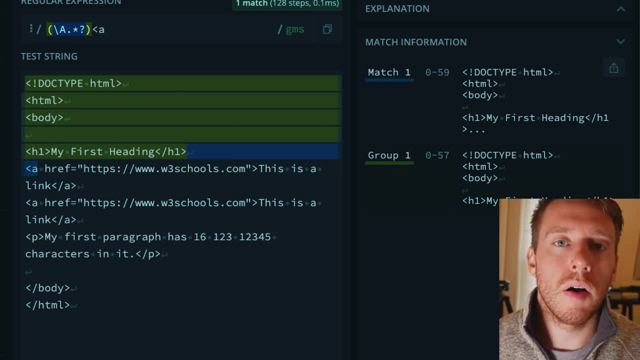 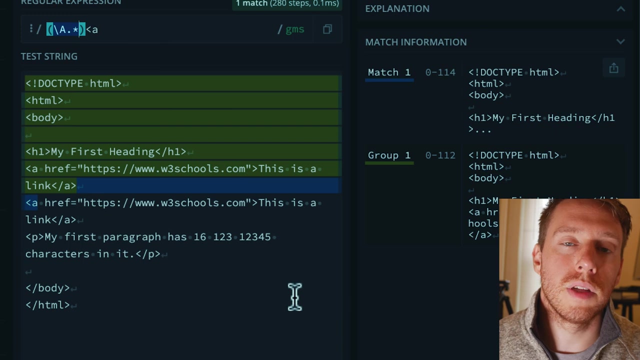 instance of the anchor tag but say i wanted to get all the text up to the second instance of the anchor tag, i would just have to remove the question mark to make it greedy, and then we would actually include that additional text. and now you can see we're going up to the last instance of the 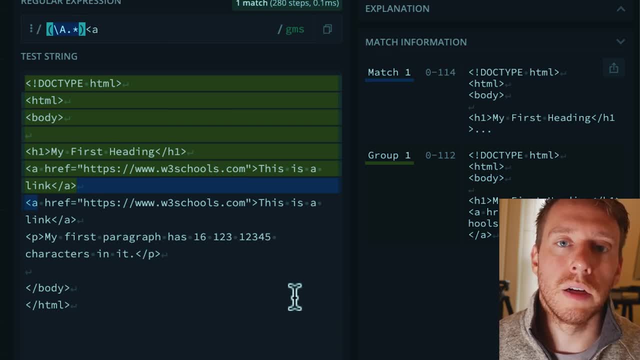 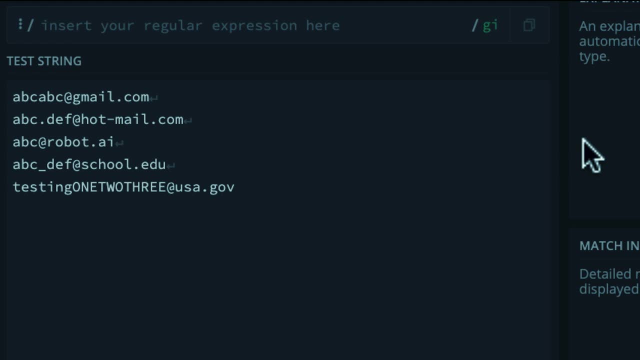 anchor tag. so just keep that in mind when you're writing your regular expressions. okay, and then one thing i quickly want to gloss over. i don't think it'll be used very much, but there's a concept called back reference. so say, we create a sub expression with a capture group that looks for a, b, c. 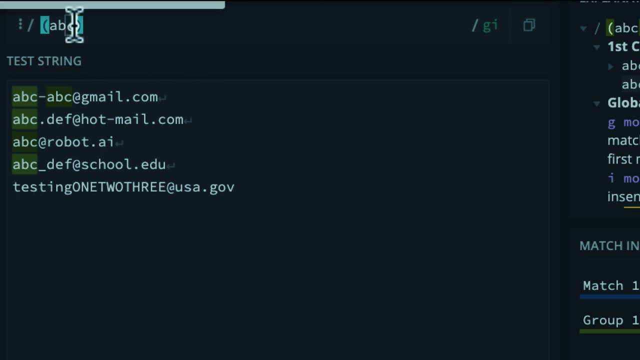 um, so it's looking for: uh, actually- sorry, let's make it more generic- let's just look for, uh, three letters and three letters followed by a hyphen, just to make it more specific. so say, we're looking for three letters followed by a hyphen, but then we want to check later on if that same exact expression, whatever- matched so in this. 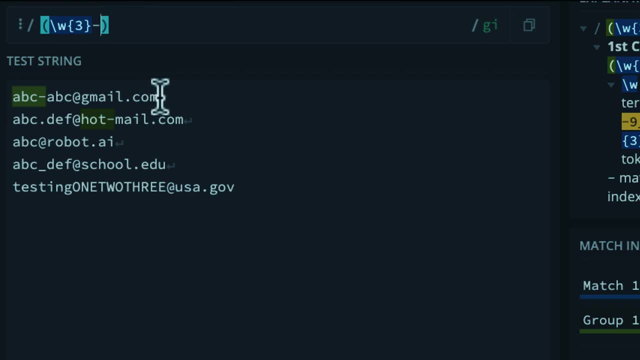 case it's a b c hyphen. say: we want to check for a b c hyphen later in the regular uh, later in the string, but we don't know. it's a b c hyphen. we only have this pattern here. well, you can do that by. 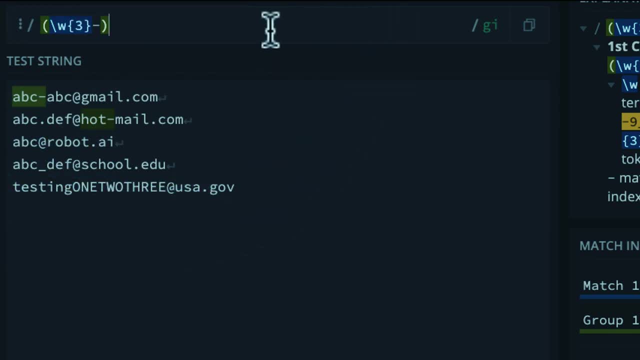 referencing the capture group as a back reference, and the way you do that is you're going to want to do that- is you do backslash index. so so say, we want to then check if that shows up elsewhere in the string and actually let's just throw it in the string so that it does in fact match. 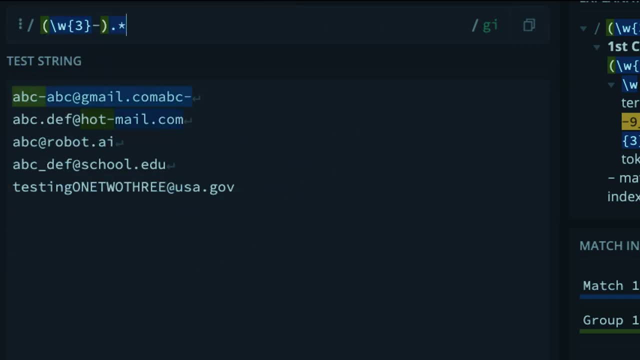 um, we can do that. so we're going to do dot star question mark and then we're going to look for the back reference. see, we're saying: look for three letters followed by a hyphen, anything in between leading to the same expression, exact pattern. and we do. and that criteria does fit this here, because we have a b c hyphen. a b c hyphen. 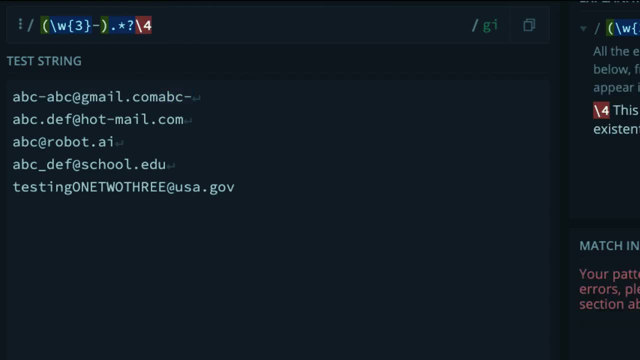 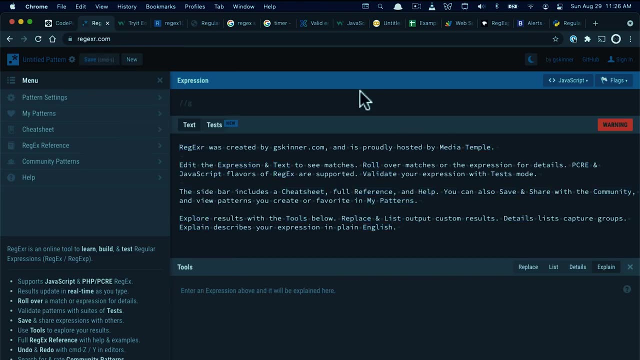 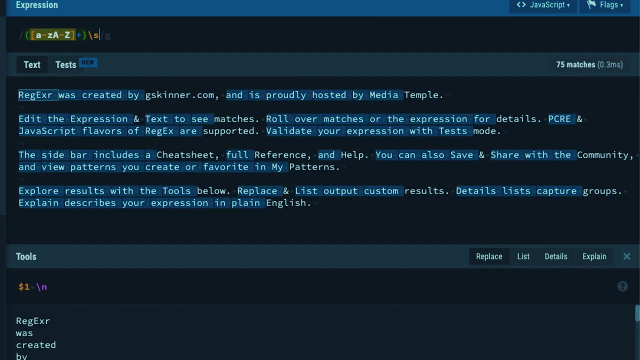 and as you have more capture groups, you would just change the, the uh, the index on the back reference. okay, and then i just want to show you how to use the capture groups. the other tool doesn't really display that very well, but let's just modify this. let's say we want just the uh, we want the first. 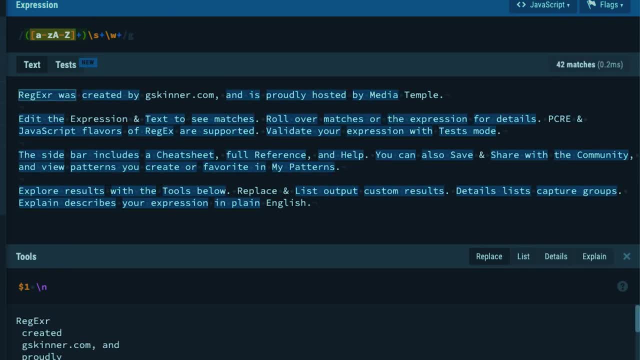 three words, so we'll anchor it to the start. okay, um, and actually we want the next word and we'll get rid of this complex guy here. we'll just do backslash w plus, all right, and then we're capturing each of the words in a capture group. 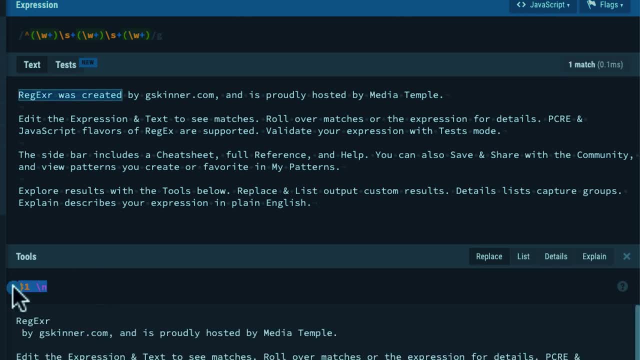 and then save. i want to rearrange them, i want to reverse them. dollar three, that's the third word, right? dollar two, that's the second word, and then dollar one, and so we can put it in any order that we want. so again, word one, two, three, regexer was created, and then we're reversing it. created was regexer. 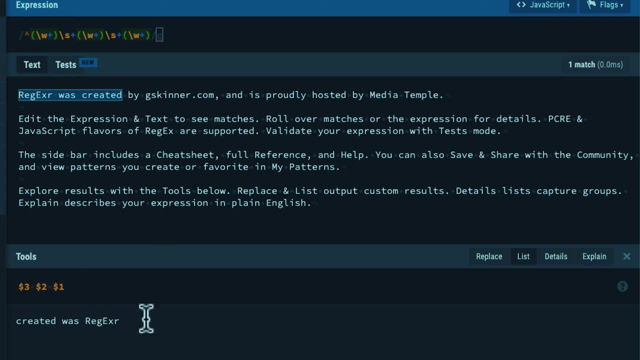 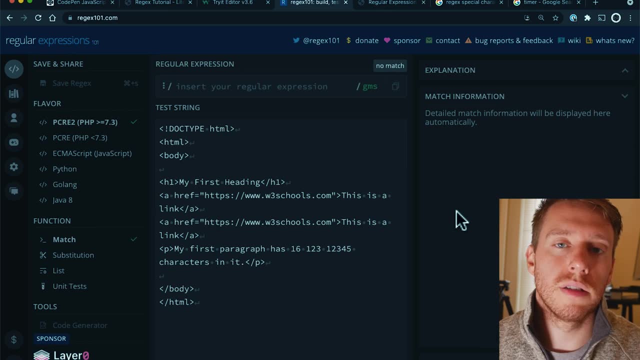 so that's how you use actual capture groups. it's usually in the context of search and replace. okay. next is probably the most advanced concept, which is positive look aheads and negative look arounds. so positive look ahead says: find a regular expression that is immediately followed by some other expression, but only include the initial. 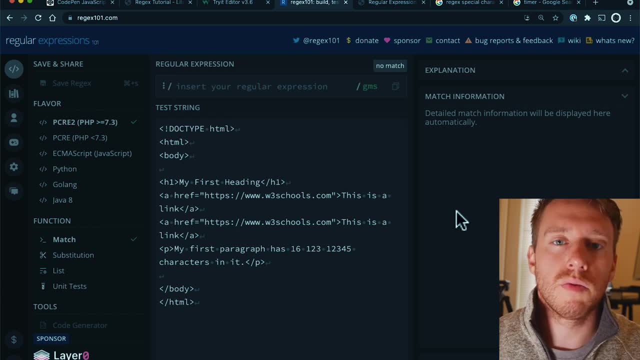 regular expression in the matching. so say, for instance: we wanted to match on any letter that is followed by a white space, but we only wanted the letter to be part of the regular expression itself. we can do that using a positive look ahead. so the positive look ahead is denoted by a capture group with a question mark and an equal sign. 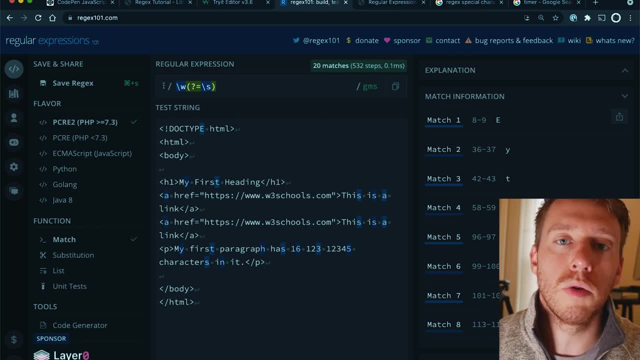 and you can see that this pattern is matching on letters that are followed by a space. so that's the qualification, but it only matches on the letter itself, not the space. next is negative lookarounds. if you want to create a regular expression that says match on text that is followed by a space, 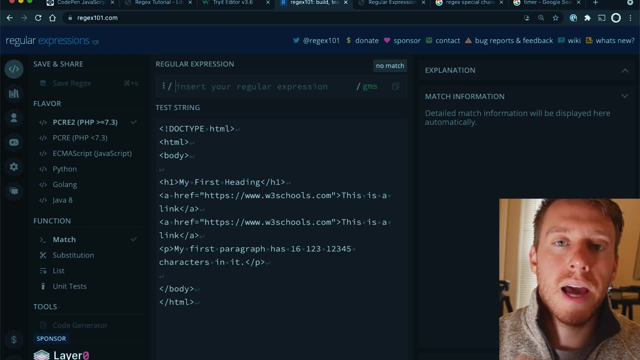 then you can do that using a negative look around. if you want to create a regular expression, that text that does not contain some subtext, that's where you want to use negative lookarounds. so the negative look around is denoted by the question mark and then the exclamation point, and what we're 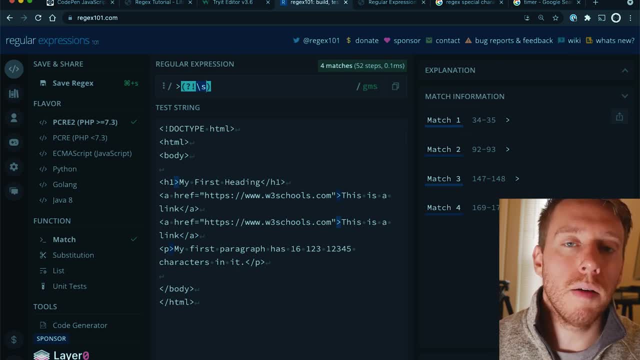 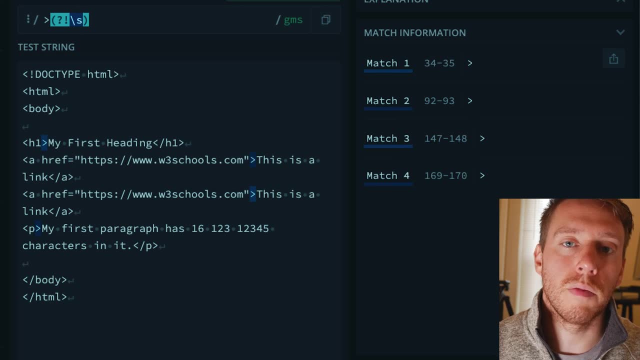 saying here is: look for right arrows that are not immediately followed by blank white space. so, as a result, we only capture those right arrows that are immediately followed by another character and not a white space. now, if we wanted to say does not contain, i'm going to show you that regex, i know. 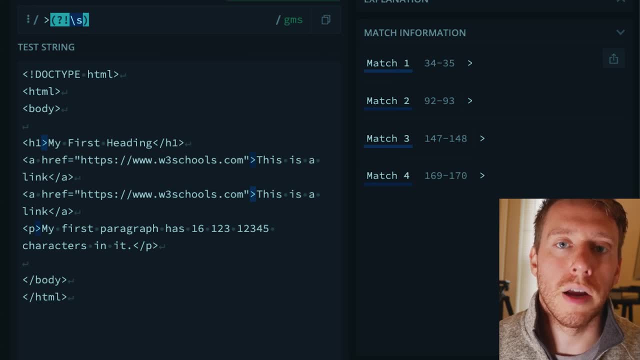 it's going to be kind of intimidating, but i will show you how to do that. so say, we wanted to match on any line that does not contain the phrase html. we can use a negative look around to accomplish that. so we'll start by using the start of line and end of line anchor and then we'll use dot star. 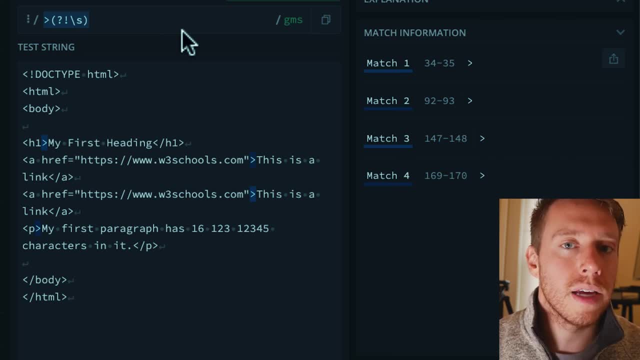 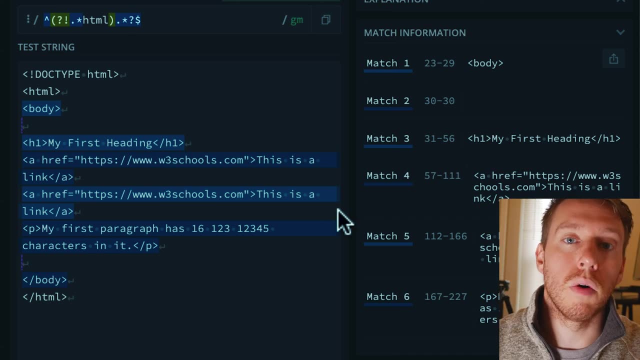 question mark to match on anything, and then we'll use the negative, look around to say, but does not contain html. okay, so now you can see we're matching on every line that does not contain the word html, and this is really, really useful. and again, we can expand this out by creating a sub capture. 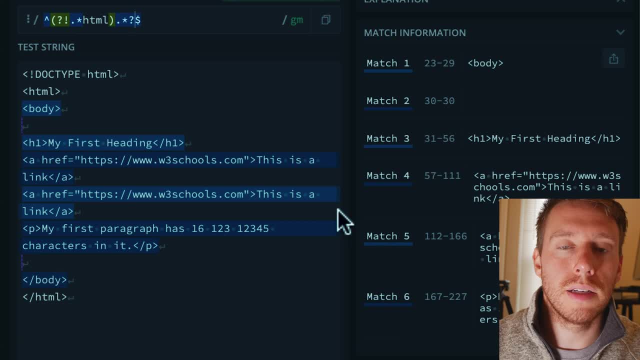 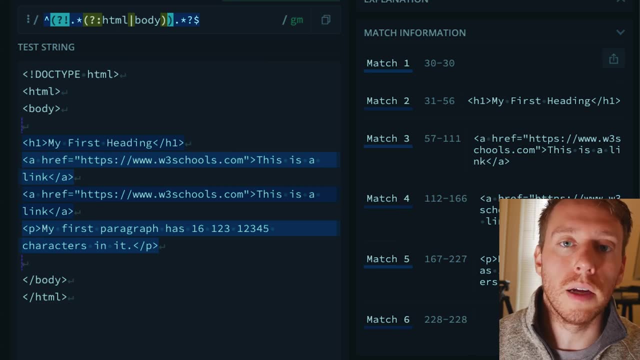 group and what we could do is we could say any line that does not contain html or body, and now you can see we're only matching on lines that don't contain html or body. this is a really useful one to have. it might be something you have to copy and paste, but it's good to be aware of this one. so 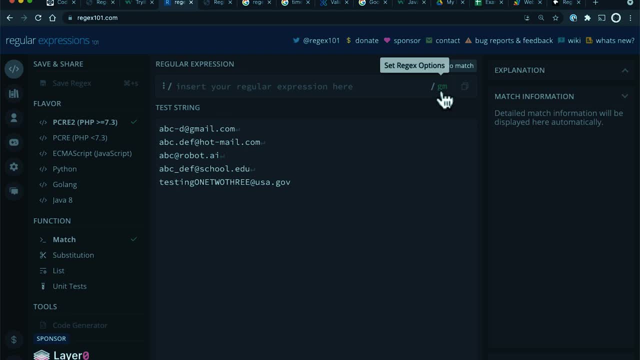 the final thing we did not talk about yet are the flags or the modifiers. so the biggest one, i think, is global and i, for case insensitive, say we want to match on any letter and we want to do that using a through z in a character class. this matches on the first instance, but if we add a flag to make it, 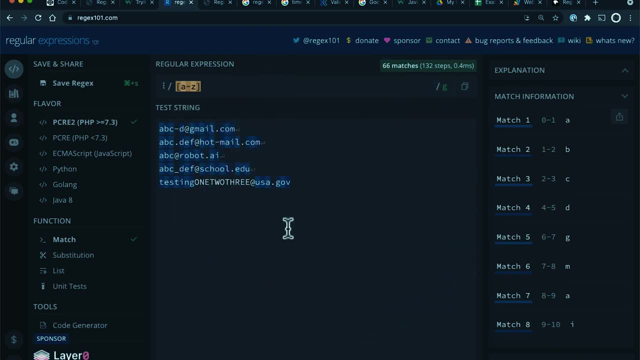 global. now we're matching on every instance, so i basically always want global. if we wanted to include, if we wanted our regex to be case insensitive, we can just go ahead and add the i flag to it, and now it's case insensitive. and so i think there are a number of different flags, but really those are the most important. 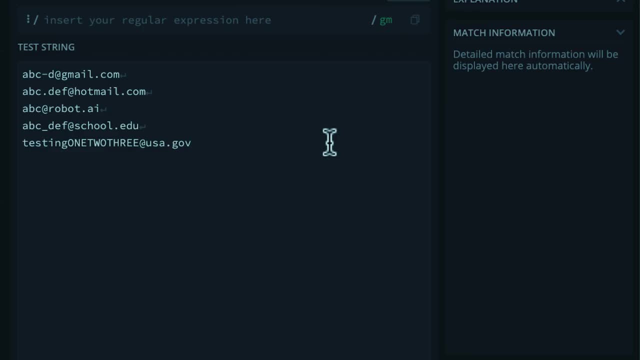 for most use cases. okay, so let's do like a real world example here. so say we wanted to construct a pattern that matches on email addresses. how would we go ahead and do that? well, we can use some of the key concepts that we just came up with. so the first thing is: every email address. 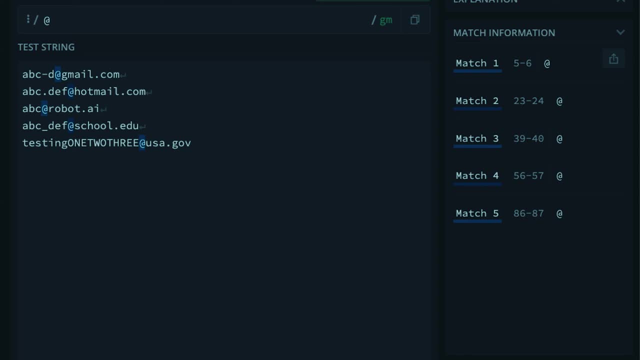 has to have an ampersand in it, right, so we can start with that and then it's followed by a domain name, a domain name, a period and then a top level domain. so for the domain name things, a domain name can have any letter or number in it, so we could do something like that. 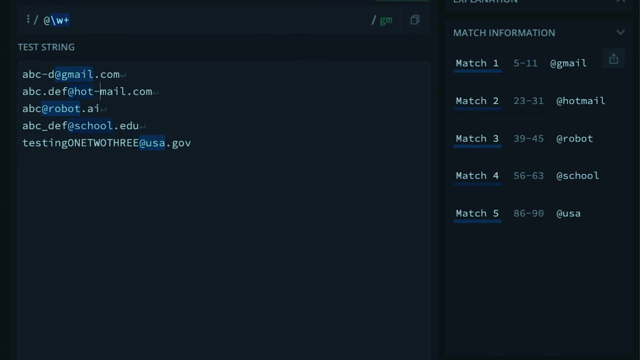 but i guess, what if the domain name had a hyphen in it and then we no longer be matching. so why don't we just do it super generically and do dot star, question mark, and then we'll do a literal period. so now we're matching on anything, uh, that's followed by a period, because we know that's a. 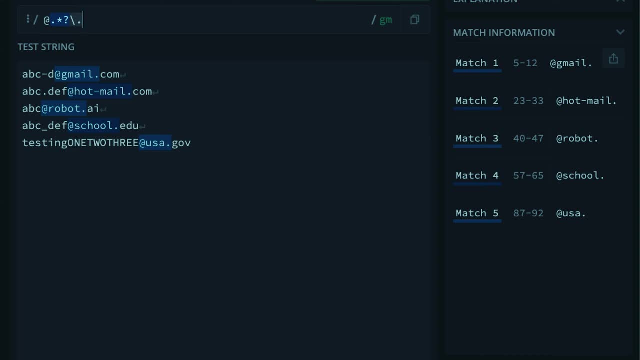 requirement and now we just have to match on the top level domain. so i believe top level domains are fairly rigid in that they are always characters, um, but they could be different numbers of characters. so why don't we just do backslash w plus for that, and i think that will suffice most. 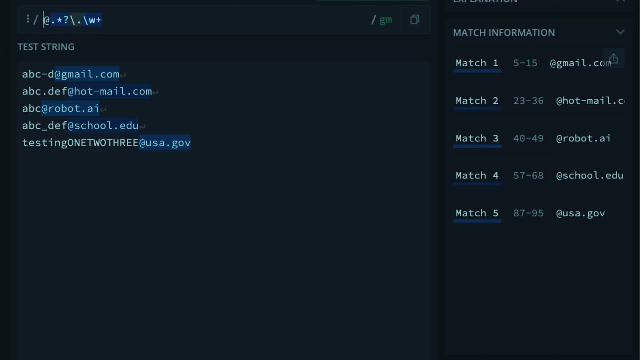 of the time. okay, so now we just need to go ahead and add the top level domain name and then we'll the actual email handle itself. so why don't we go ahead and just use- we want to build a match on hyphen special characters, so we could do something like start and then we could just do dot star. 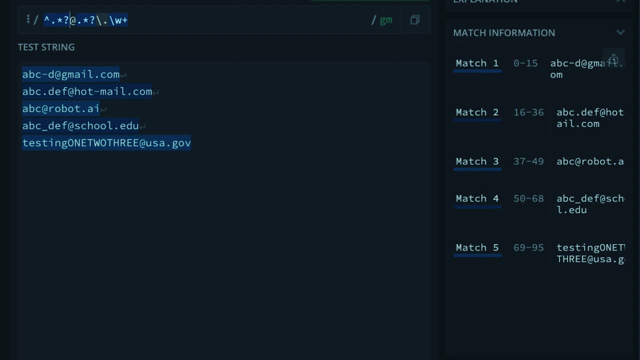 question mark, and then we'll just look for the ampersand, and so now, when we are validating a string, we can determine if it's a uh email address or not. now, this is not perfect. this is what i just came up with very quickly, but this, this is something that you might actually 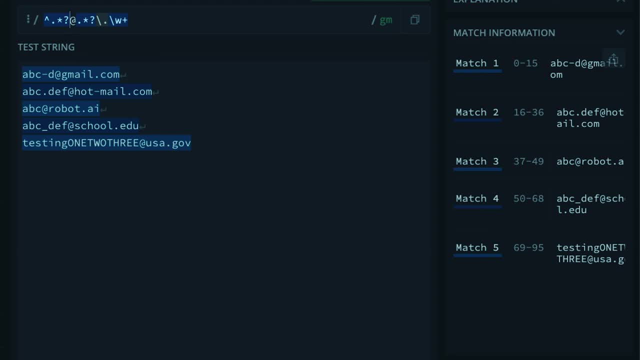 write with real code when you're building an application. so now that we've done a bunch of examples of constructing regexes, let's actually dive into some real world use cases and get our hands dirty with some actual code, and we're going to see how this is actually implemented with actual 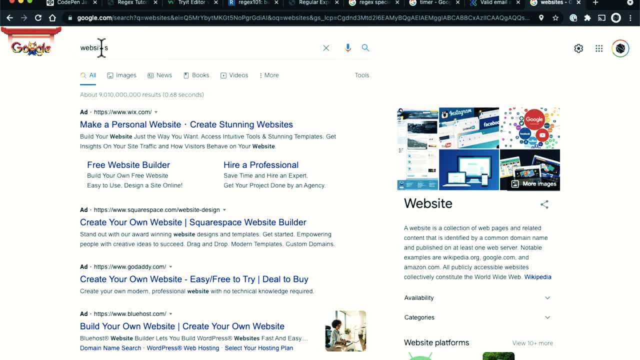 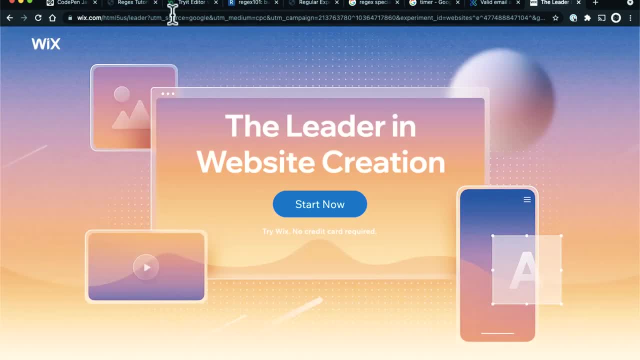 code examples. so i'm going to go ahead and just search for websites and i'm going to click on one of these ads here, and the reason i'm going to do that is because when i do, there's going to be these url parameters that are passed in the url that denote various marketing campaigns and what i want to do i'm. 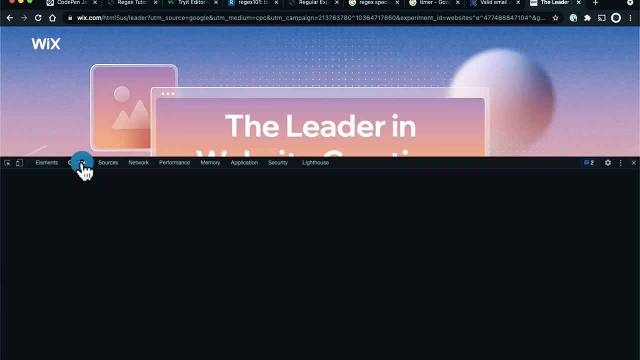 going to pop open the javascript console here and now. we can write some code to maybe extract these url parameters here when we're writing a regex with javascript. there's two ways to do it. one is you can use a regex object, the second is to use a regex object and the second is to use a. 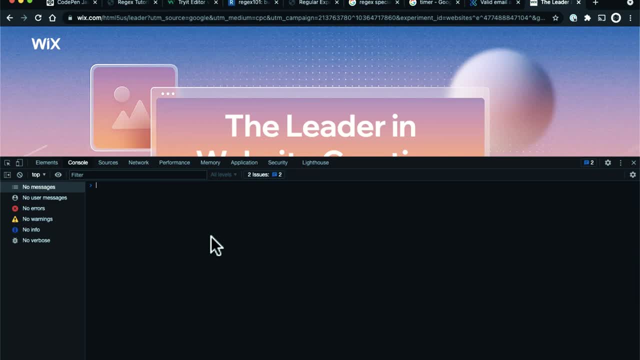 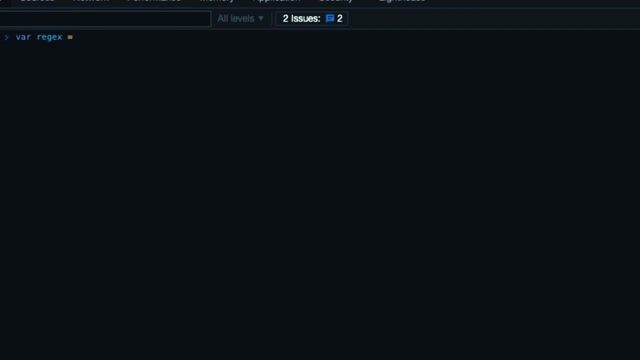 literal string as a regular expression. so let's create our regex real quick. and now there are different functions that we can evaluate against the regular expression. so one thing we want to first do is just grab the url. so i'm going to do var url equals windowlocationhref, and just so we can ensure that we have that. 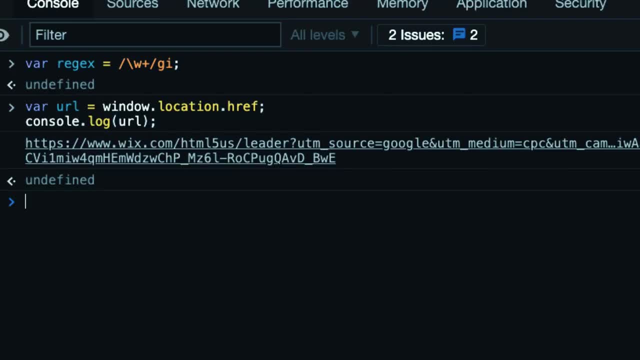 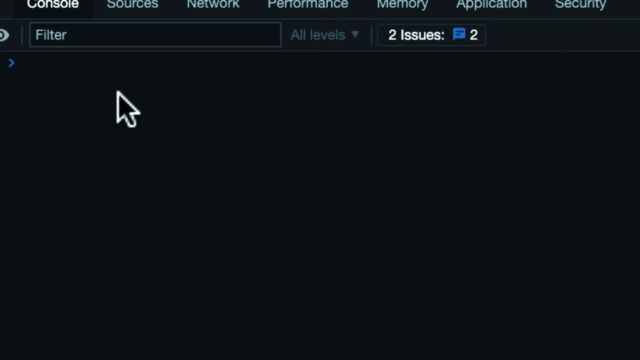 we're going to go ahead and log it to the console, and we can see there that we do in fact have the url including the query parameters. so now let's combine these two and run a regular expression against the url, and match will return an array of all the different instances where 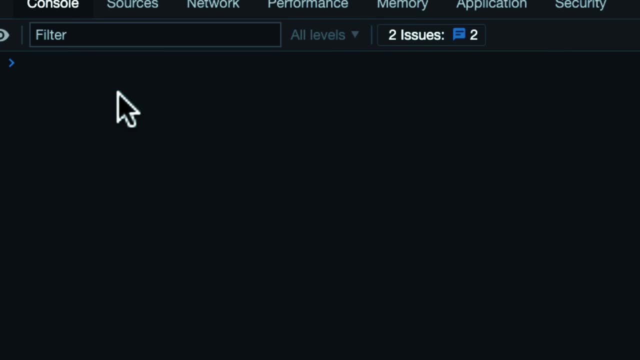 that regular expression was found, so let's go ahead and use that. so again, i'm just going to do window dot location, dot href, and then i'm going to do dot match and we're going to pass in our regular expression. so again, we could just do backslash w plus, and now we are getting an. 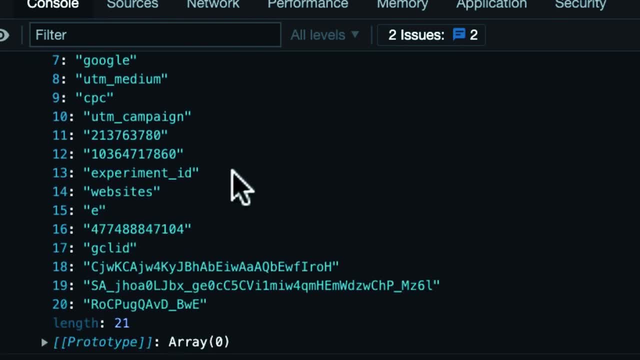 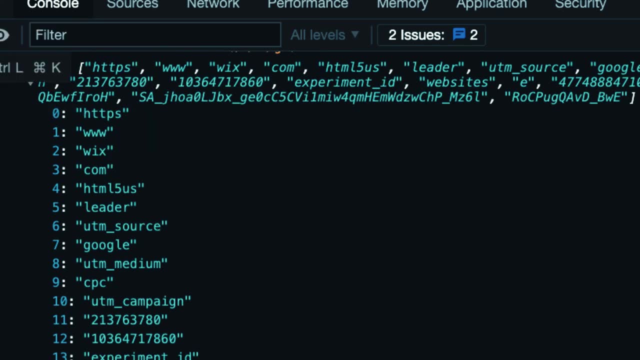 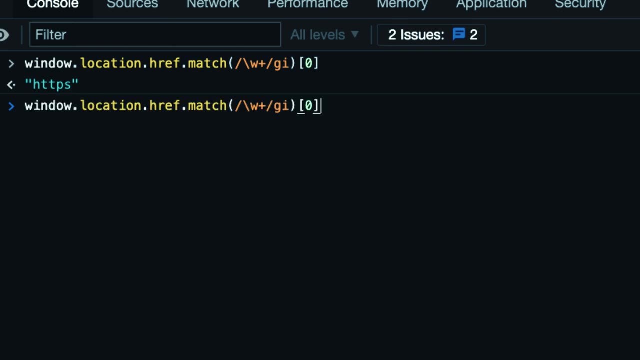 array of every single instance of essentially- uh, kind of like a word phrasing. so, and then if we wanted to grab a particular one- so say, for instance, we only wanted the protocol- we could just index it as zero. and we're only grabbing the protocol there. now we can also. 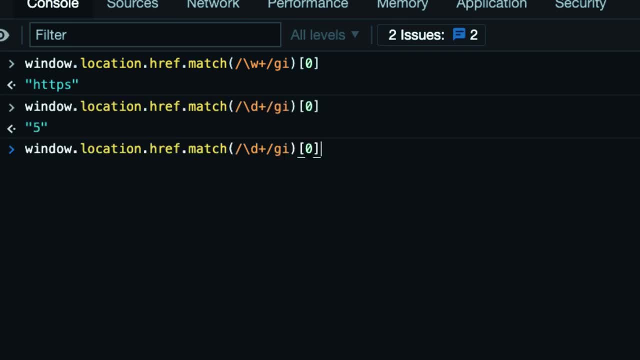 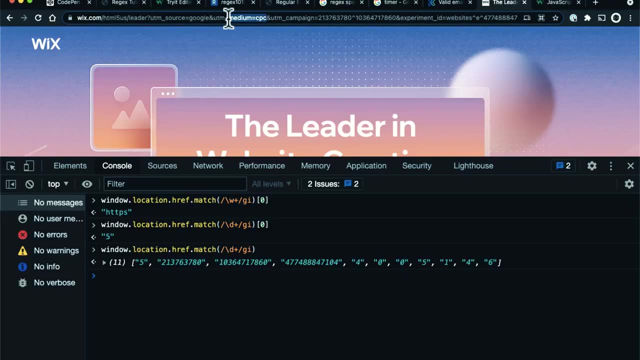 create different regular expressions, like maybe we don't want to grab all the digits- and we can do that as well and it's super easy- but say, we want to grab the parameter utm, underscore medium and we just want the value, because url parameters follow a name value key pair. so we 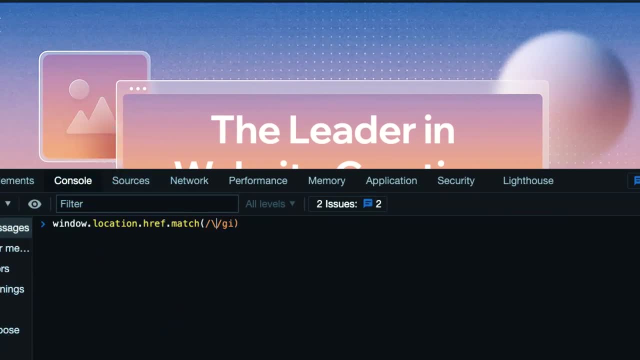 just want the value. so what we're going to do is we're going to say: look for utm, underscore medium, followed by an equal sign, and then there's different ways to get the next word. we could do backslash, w plus, so this is now capturing the entire regex, but we only want this substring here. so that's where. 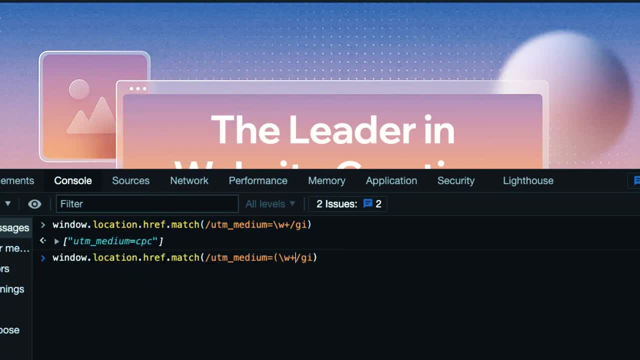 capture groups come in. so we're just going to throw a capture group around this and actually for the capture groups to work, we just have to remove the global, which is fine, and now the returned match is going to be the first index in the capture group. so 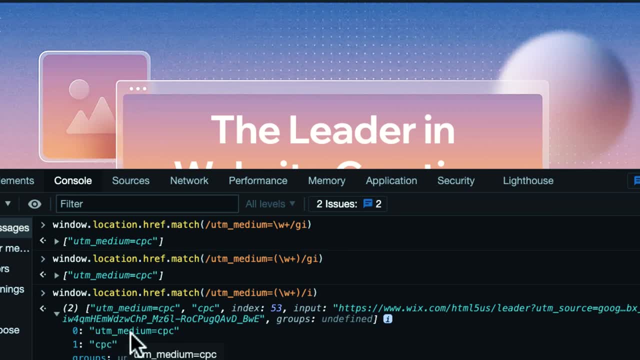 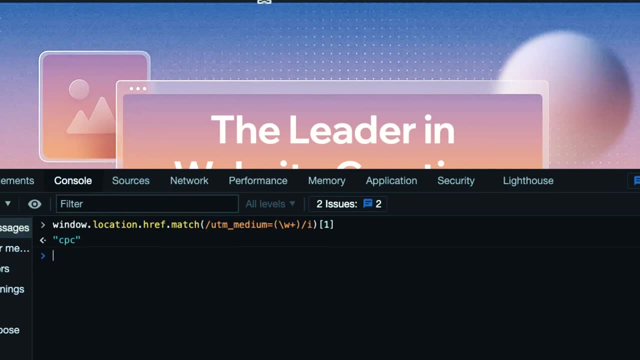 if we don't, we're still getting an array, we're getting a match of the regular expression and then we're getting the capture group. so so with the single line of code we're able to extract all the utm underscore medium campaign values. so you can see that's pretty powerful. now here's one. 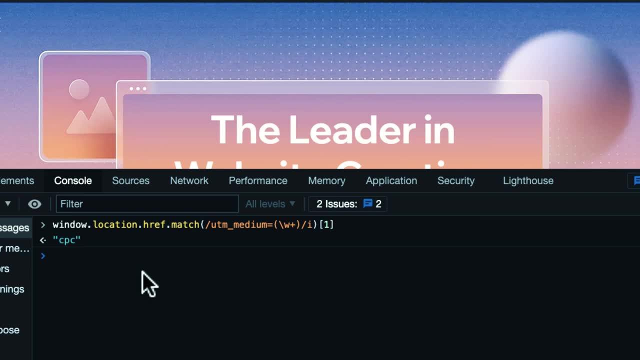 other thing that's good to have in your repertoire. a lot of the times when folks are writing code and they want to determine if a string contains a substring, they use index of. so, for example, they might do something like window dot, location dot, href dot, index of and then they pass the substring. so maybe they want to check if. 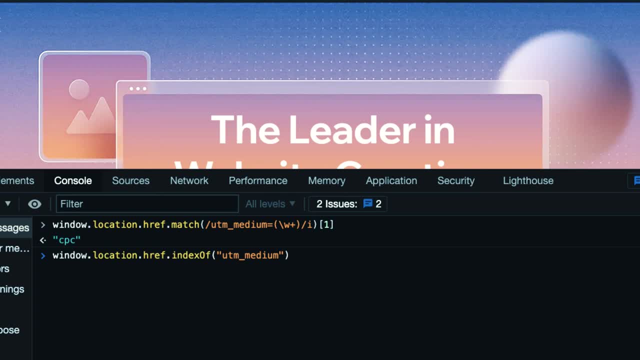 you know, utm medium is in there, and if it's not in there, um, it will return uh, negative one. so like, if we, uh, if we change the phrase to utm not found, it returns negative one. and then in their if logic they say greater than, or they just say not equal to negative one. um, they can determine. 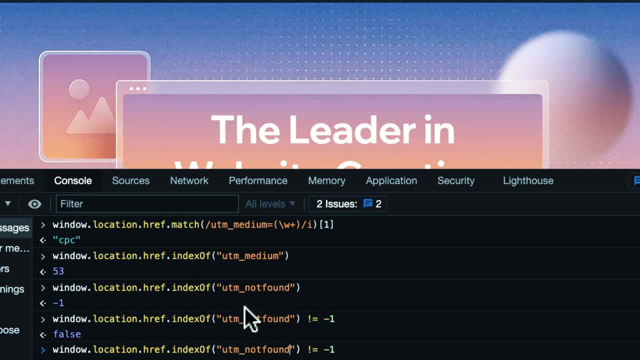 if, uh, if the string is contained within the, if the substring is contained within the string, well, this is actually not the right way to write this code. the right way to do it is to use a function called test, and it's more concise. so the way you would actually want to do this is you would write: 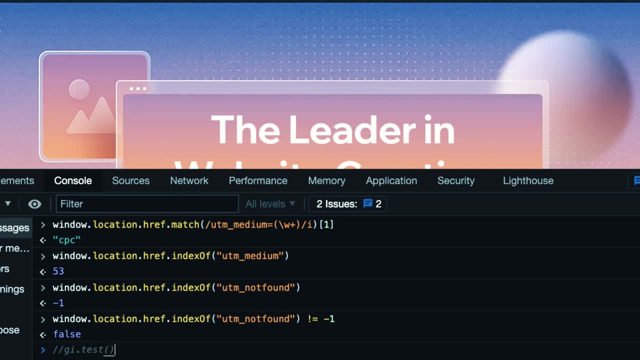 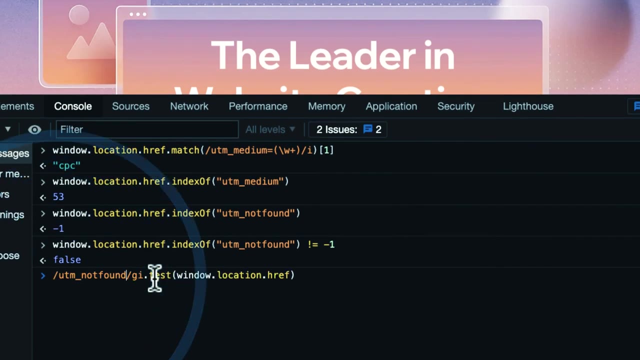 a regular expression and then you'd run the javascript method test against the string. in this case it's window dot, location dot, href, and then the um, the string that we are, the regular or string that we care about. we would just pass that in like so, and this will always evaluate to. 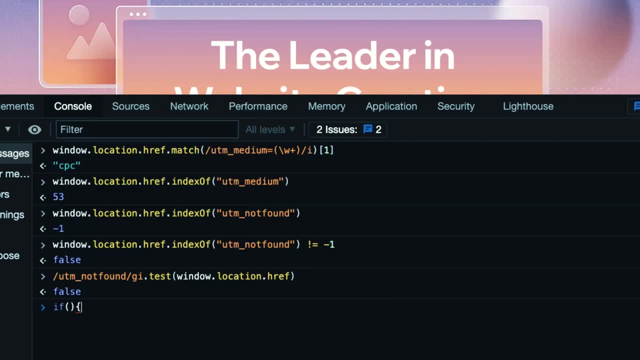 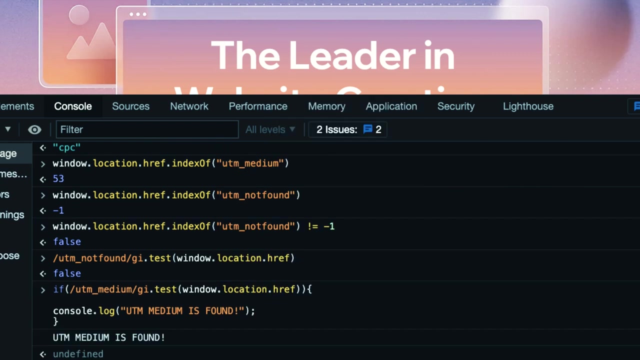 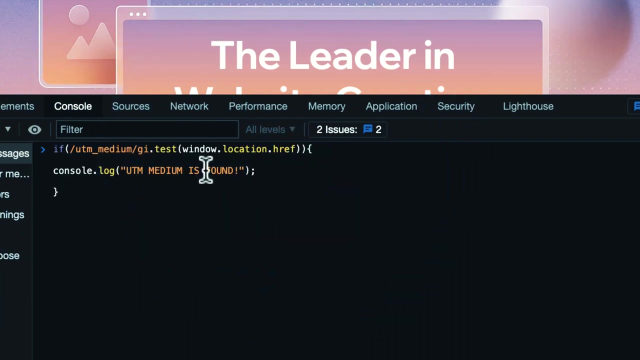 a boolean. so again, if we wanted to write code that said: um, you know, console dot log, utm medium is found. the way you properly write that is you do a regex and then against the text test string, and that's how you do that. and if you wanted to say not found um, so say utm medium is. 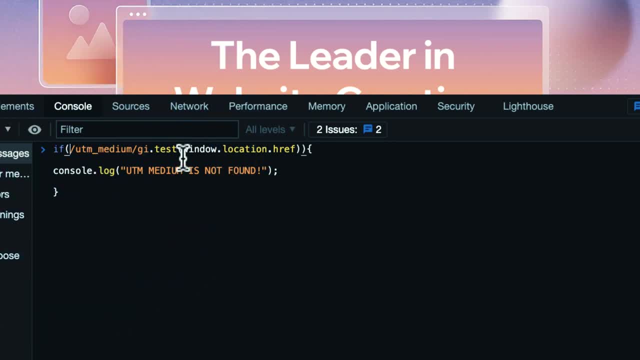 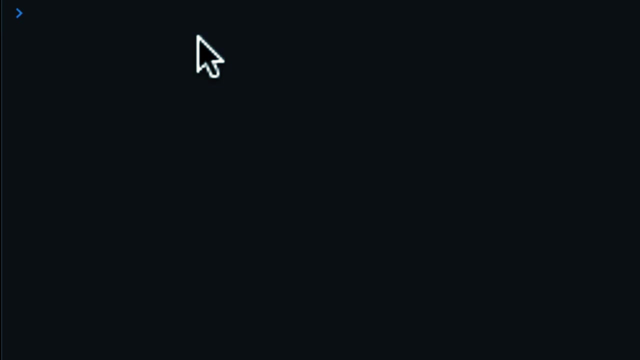 not found. you could just invert the regular expression by prefacing it with a exclamation point or bang. so this evaluated to false because we do in fact have utm medium and that's the better way to check for substrings within strings. okay, so i want to show you one more way you can create. 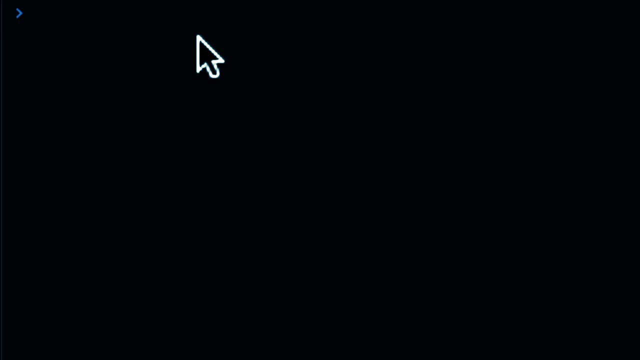 a regular expression in javascript which is to use the regex object. so we could do: var pattern equals new regex, and then the first argument is the regular expression itself, so we could do any letter, one or more. and then the second argument is the flags. so we could do gi for global case and sensitive, and then we can. 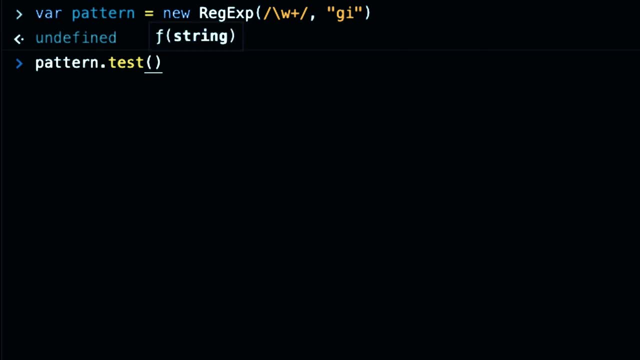 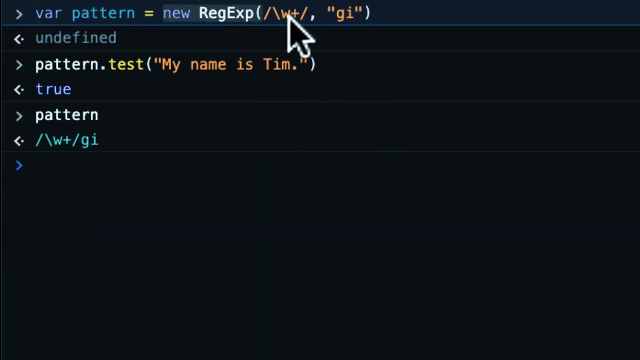 just test it using test and then we'll throw a test string in here and this should evaluate to true and we can also see what the regex is by just logging it like that, the only time i use the object is when i want to pass a variable into the regular expression. so, for instance, if i did var. 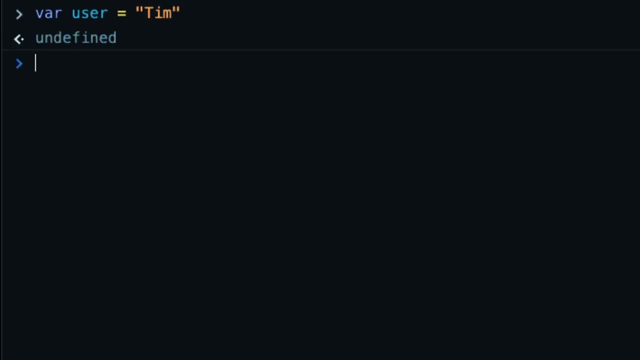 user equals tim. say, i wanted to create a regular expression out of the variable tim. the only way to do that that i know is to do is to use that regex object. so so you could do um, but say we wanted to like add something else to it. we could do um, you know. 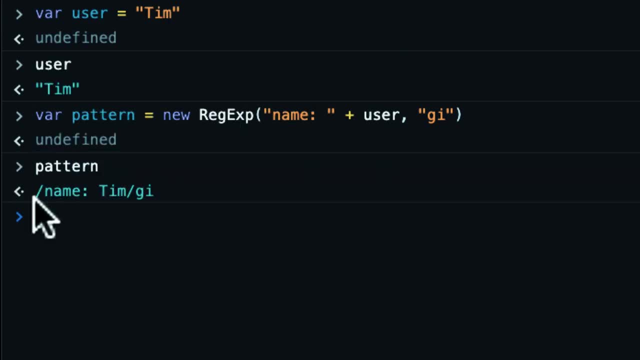 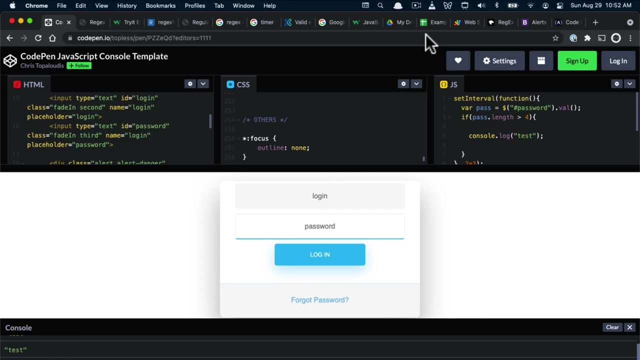 right. so that's the only way to create a regex dynamically is to use the regex object. but short of that, if i'm writing a regex, i just write it inline like this, and then you know I can test it against the string, just like that. okay, so I want to show you another example here. so we have a 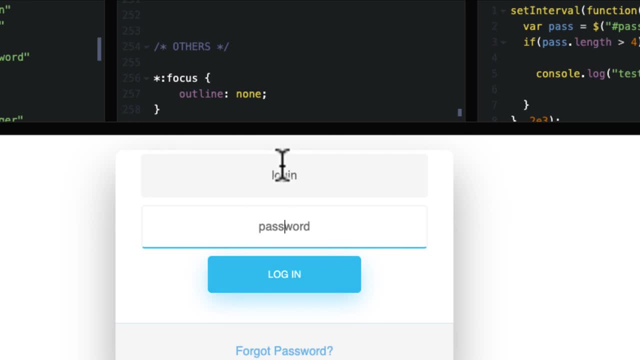 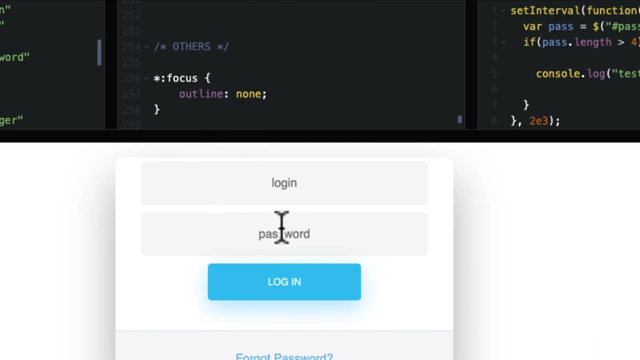 code pen script up here that is just showing a very generic input login form, and where you might want to use regex is to validate on the client side whether the password is valid or not. so if the user types in something that we know doesn't follow our password requirements, then we don't even have to send it to. 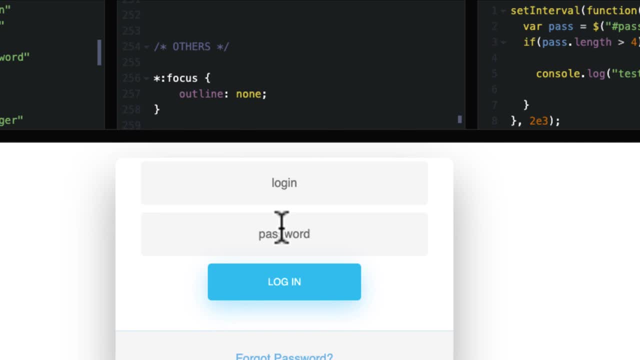 the server, we can just notify the user that the password is invalid. so that's what this code is doing right here. every three, every two seconds it's running, it's taking the password field and then, if it's greater than four characters, we will run an evaluation sequence here. so I'm just going to modify this code to 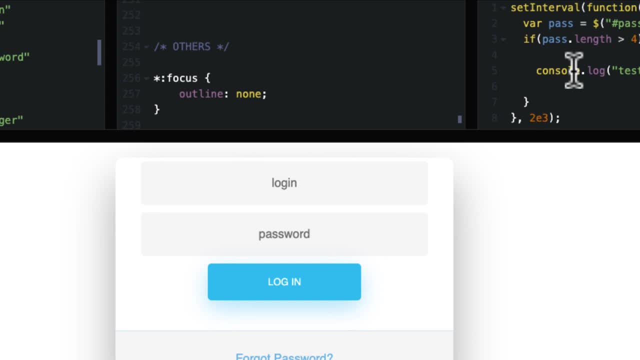 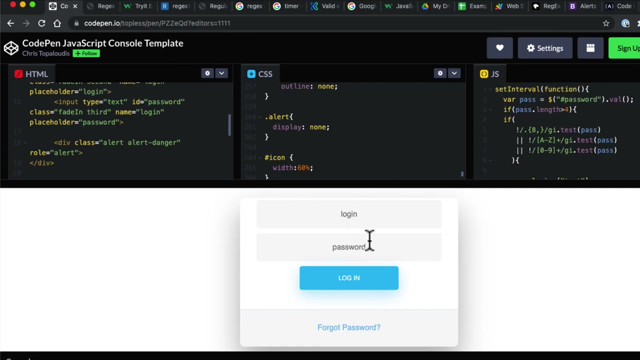 check that we have digits, that the length is greater than eight and that we have an uppercase letter, and if those are all satisfied, then we allow the user. proceed you. if they're not, then we show an error message. okay, so what I did with this code is I said: don't evaluate the password unless it's greater than four. 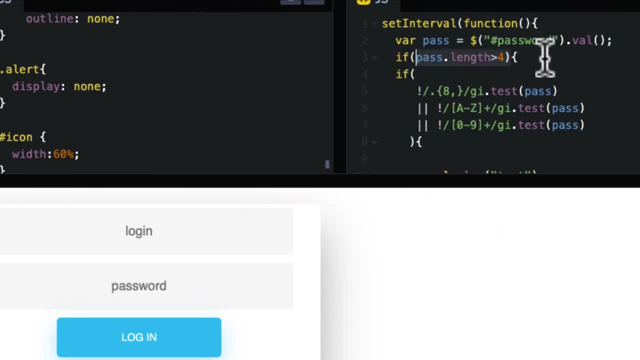 characters, just so we're not annoying the user before they've typed anything, but once they have typed greater than four characters, we check that the password is at least eight characters, eight or more characters. we check that there's a capital character, one or more, and then there's a digit one or more, and 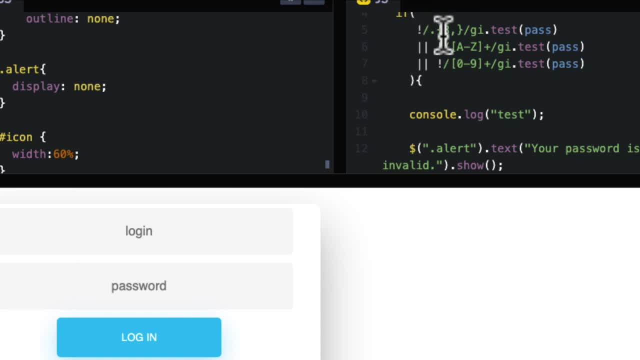 if any of those are not valid, then we will show an error message. if they're not true, that's what I put the bang in front of it. if any of them are not true, separated by the or, then we throw a validation error. so let's just do pass. 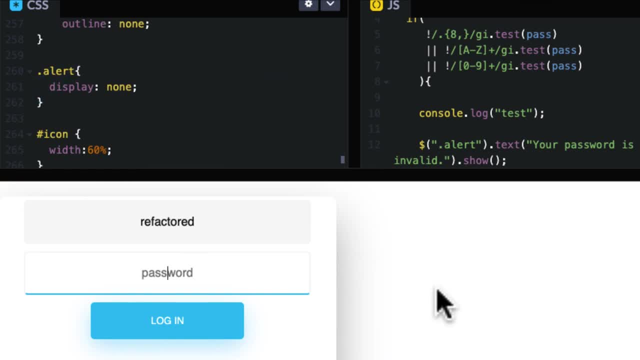 username is refactored and then password will be: my name is Tim and you can see we didn't meet the the digit requirement. we didn't meet the capital requirement. so let's see if we can't rectify that so we'll add a capital letter. that in there. so we're still out of compliance. 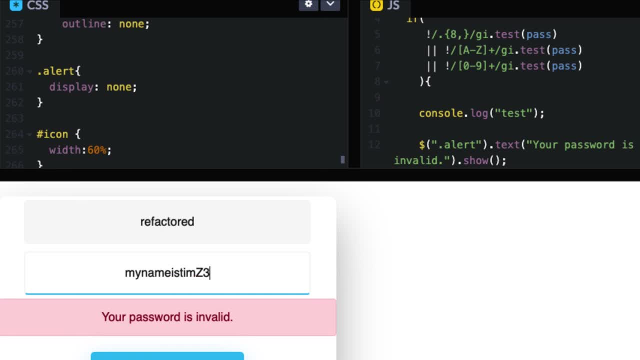 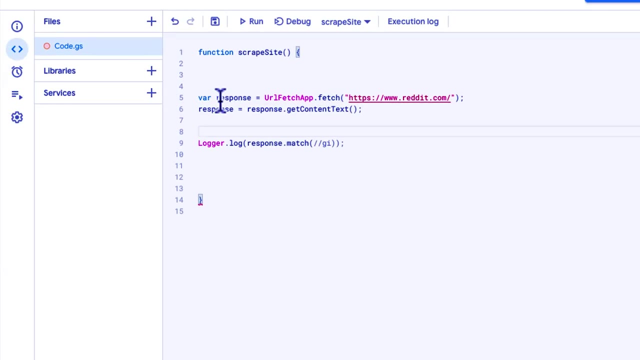 because we don't have a digit. but if I throw a digit in there then the error message goes away and we're able to proceed and log it. so you can see how regular expressions can be used for client-side form field validation. okay, so say, we want to do some web scraping, so I have an app script here that is. 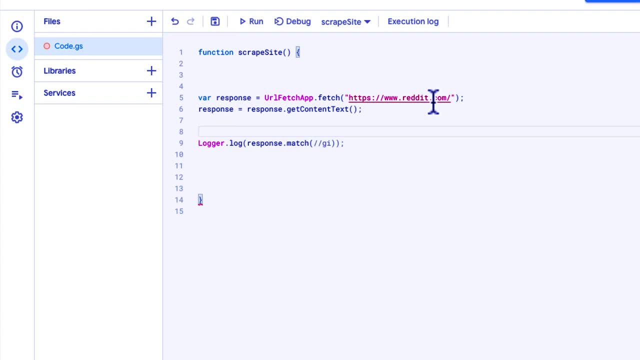 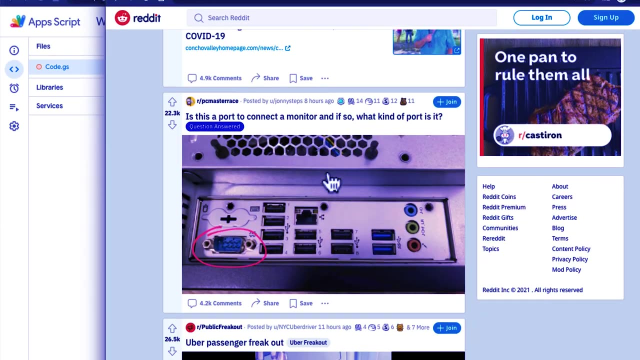 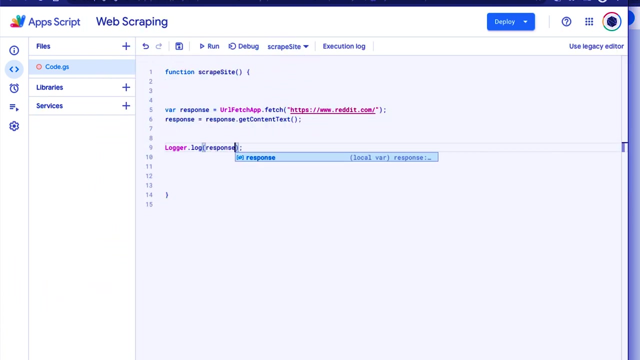 going to make a URL fetch to redditcom and say we want to get a title of the page and then we want to get the titles of every post on this page. well, first we got to see. what does that actually look like in the HTML of the page. so first we'll start off by just logging the response. so basically, 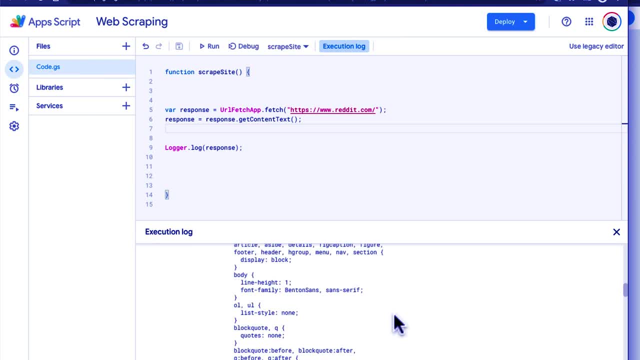 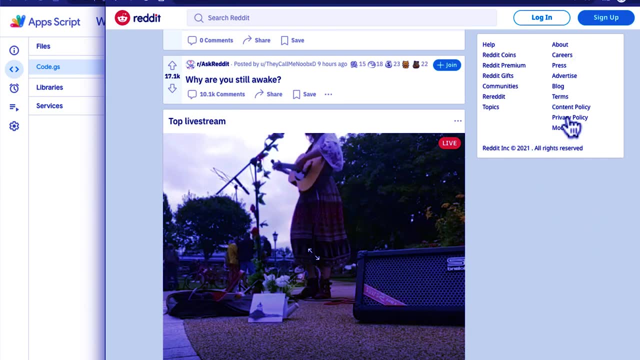 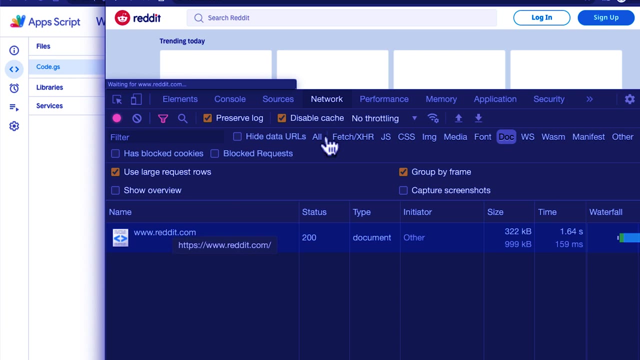 what this code does is. it just makes a request for redditcom and it logs the initial HTML source and then, from that HTML source, using regular expressions, we should be able to construct it. so I'm going to refresh redditcom and then we'll just look for. 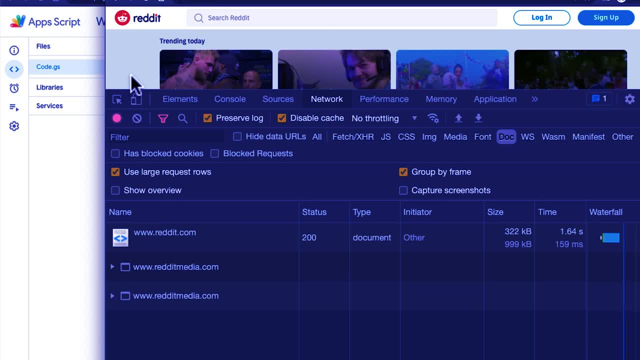 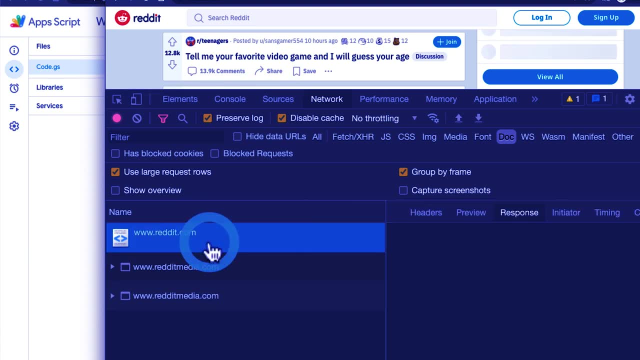 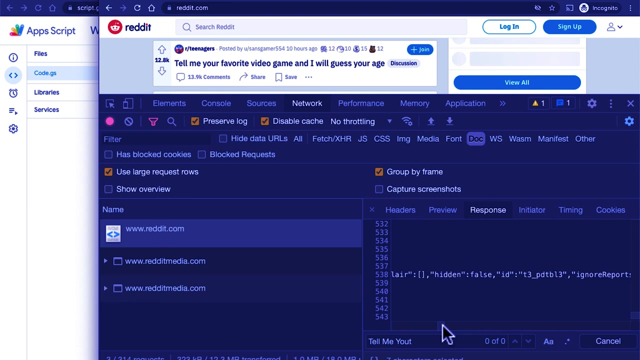 one of the type of posts- title- and then we should be able to determine what's what. so there's a post called tell me your favorite video game. so I'm just going to look in the HTML, tell me, all right. so it actually looks like there's kind of like a data layer here. 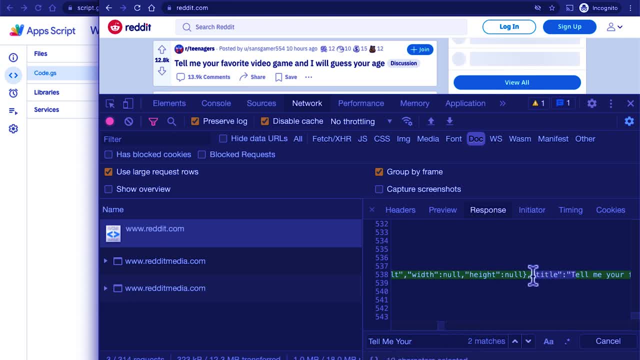 that we might be able to use. so let's take a look at this. all right, here we go. so there's a data layer that we can match on, so we can write a regular expression to find that. so we're going to come over here and we're going to say: 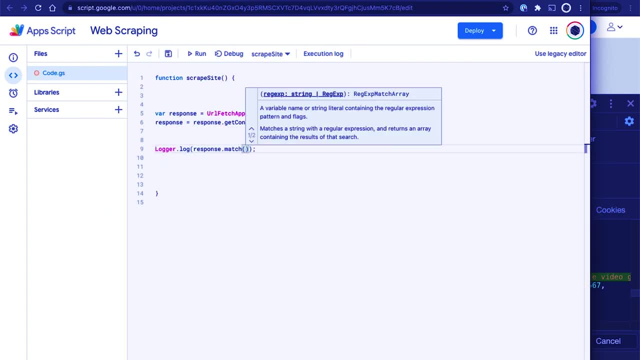 take that response HTML and let's evaluate our regex against it. so a couple things here is: I don't know if there's always going to be a white space, so let's do backslash a star, and then what we actually want is what's contained between the two double quotes. so we're going to use a negated character. 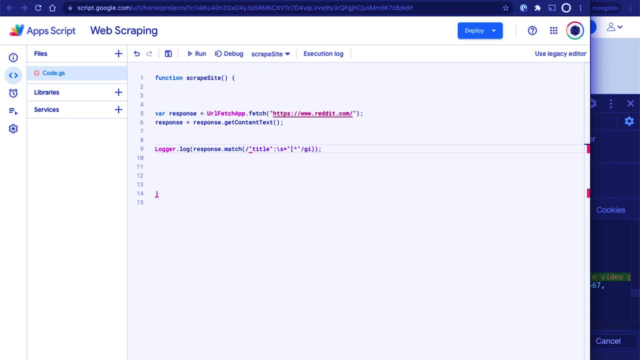 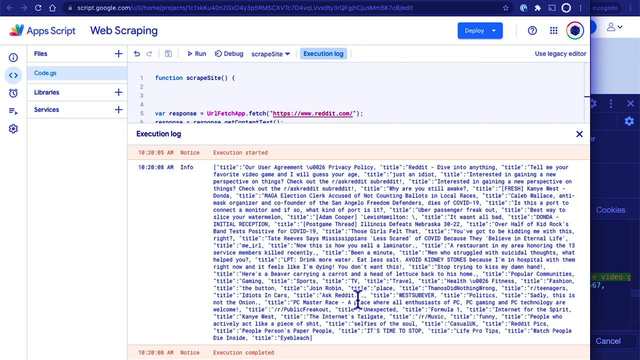 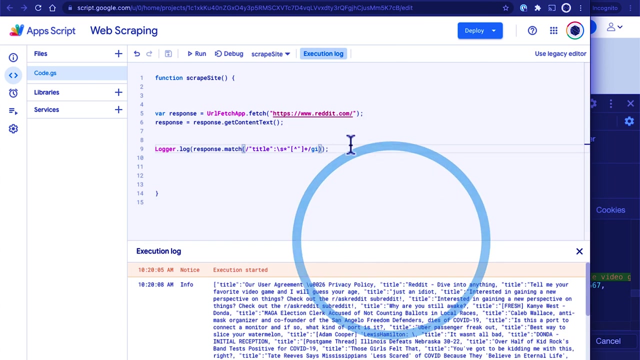 class to say match on anything that is not a double quote, and let's go ahead and see what this returns. okay, so it looks like actually we did get all the titles. so let's- um, let's just write a little bit of code to make these a little bit. 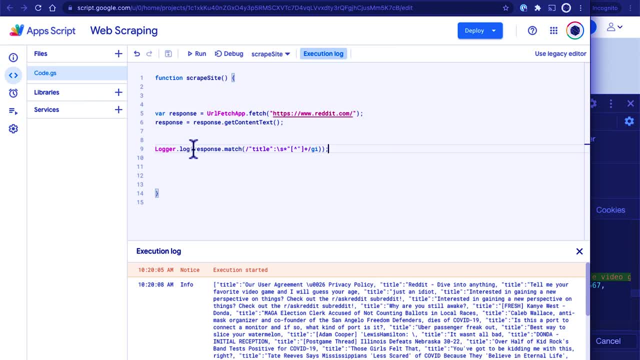 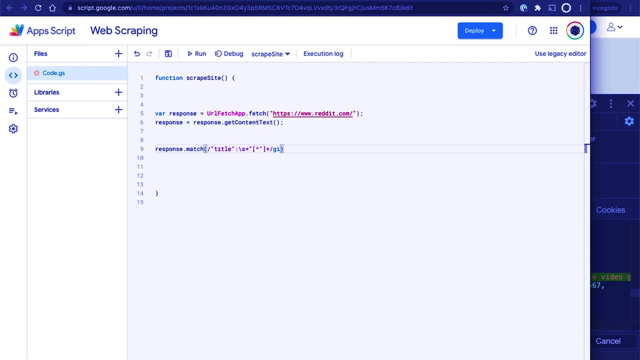 prettier. so what we're going to do is: let's iterate over some of this stuff. so this is an array and we're going to do dot for each, and we have two parts here. I forget what they're called, so I'm going to do A and B. 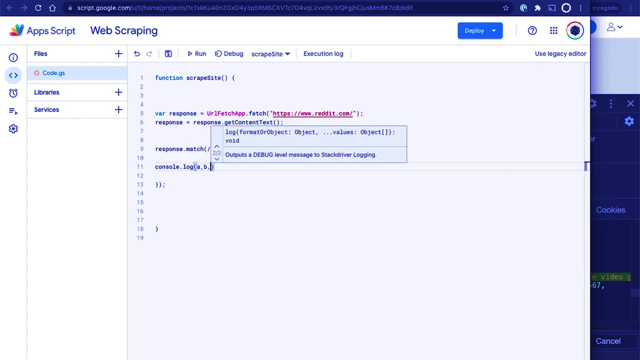 and then we'll add a new line in there and hopefully that will make it a little bit prettier. but actually we don't want console dot log, we want logger dot log because we're using an app script. let's see if this helps us read the data. 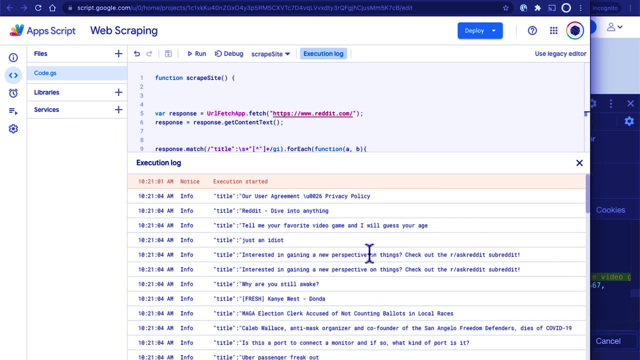 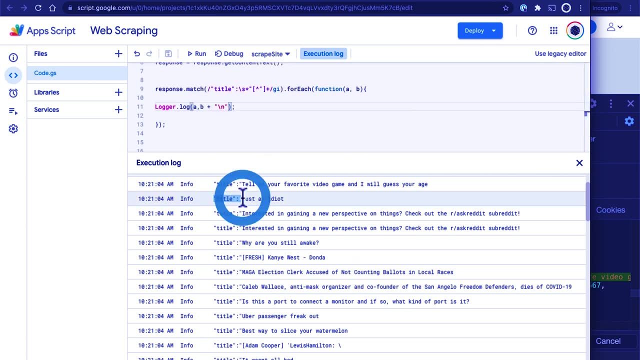 better, so it does. so this looks pretty good. so these are. these are the titles of the posts, but we don't really care about this part here, so we're going to do a little bit of code here and then we're going to do a little bit of code here. so what we can do is we can actually remove that if we. 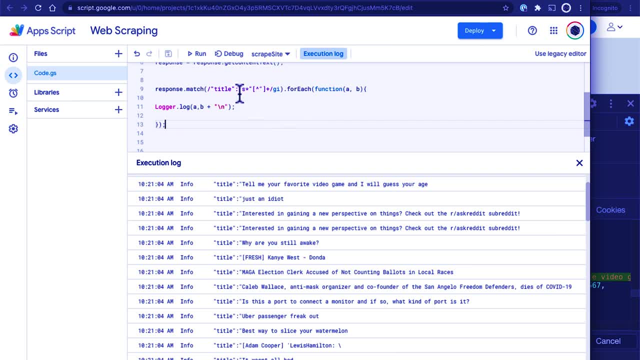 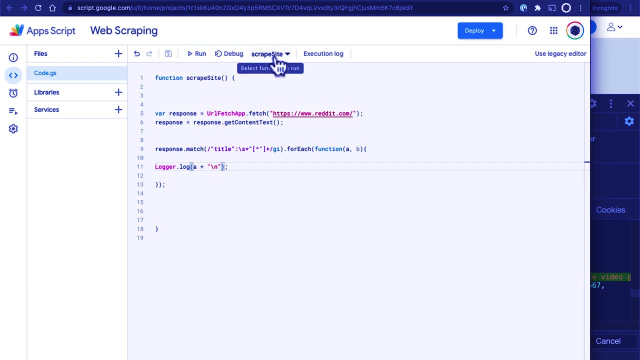 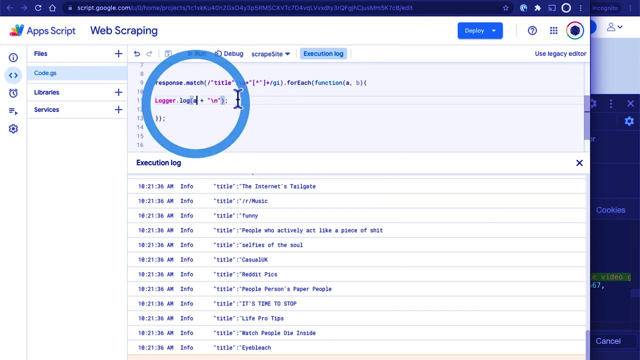 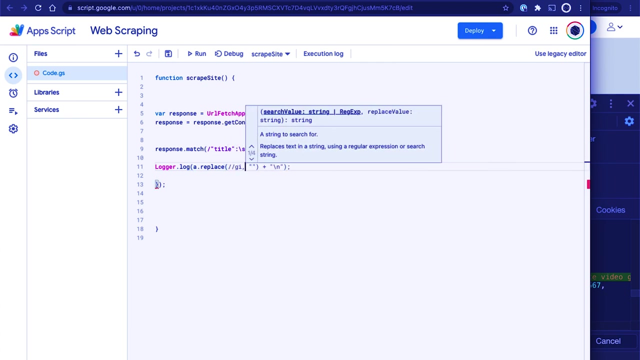 want. so let's go ahead and do the following. so I think A is the actual search term. let me confirm that. yeah, so we can use regular expression actually again to remove some of the text that we don't care about. so we're going to replace, we're going to look for a regular expression that says title. so 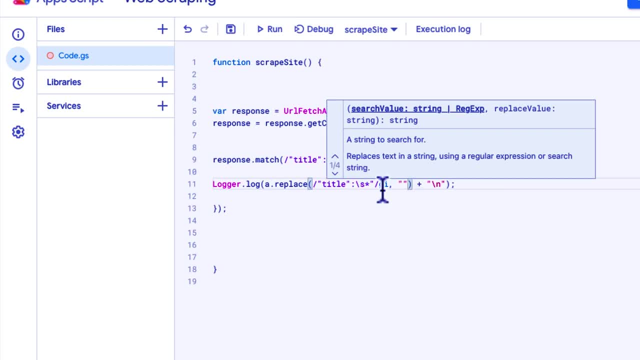 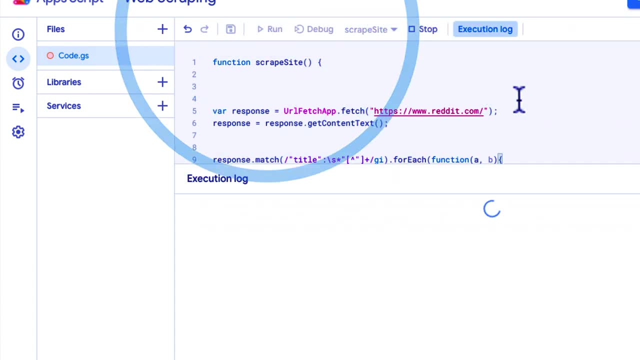 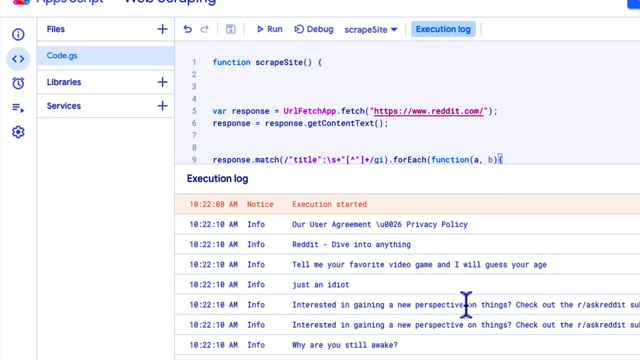 okay, so we're looking for a regular expression to match on that text that we don't care about, and then we're replacing it with nothing, so I think this is going to give us exactly what we're looking for. yep, so you can see. so not everything was a title, so it's got some other stuff in there, but tell me, 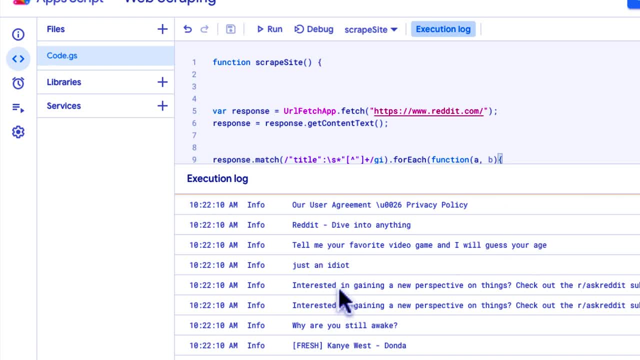 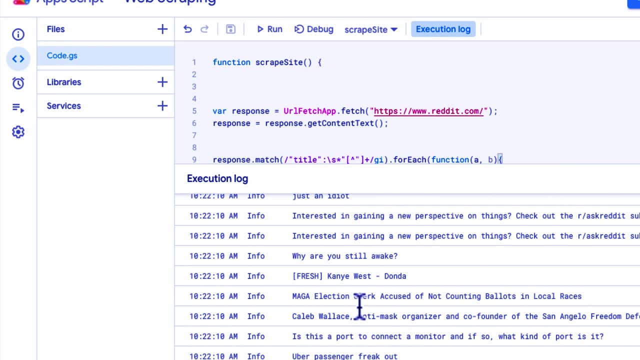 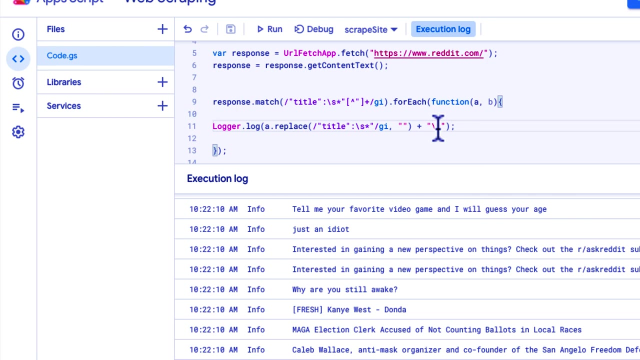 your favorite video game and I will guess your age- just an idiot. interesting, getting a new perspective. okay, and we're getting some of those titles, of those different, those different posts, so it's very easy to extract data based on a pattern from even complex or unstructured test string, such as just the HTML of a page, and then we're going to give them some additional information.